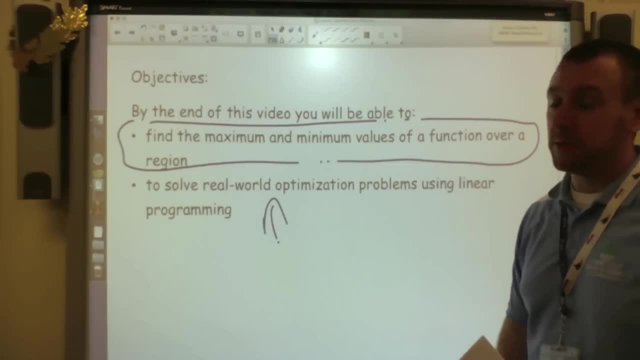 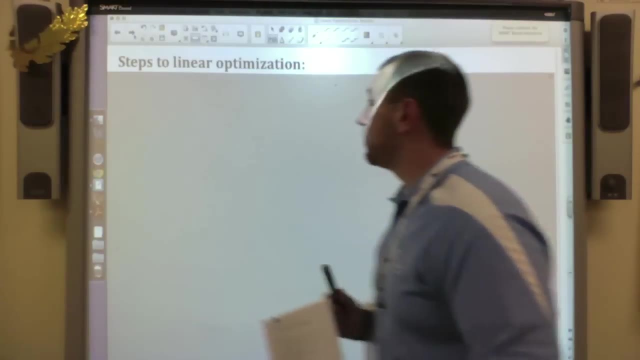 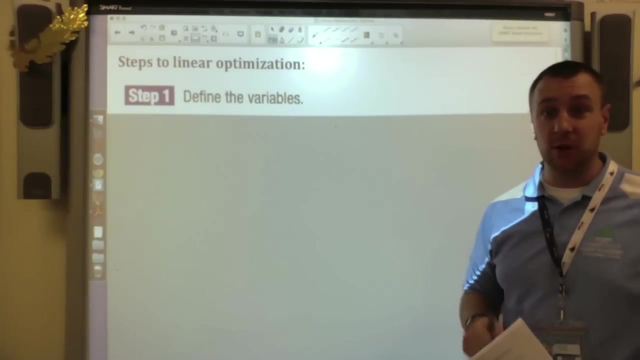 trying to help you with this and we're trying to help you with these application problems, okay. So hopefully by the end of this video, you'll feel very comfortable with that. So steps to linear optimization. okay, The first step is to define the variable. okay, And it's right in here, okay, 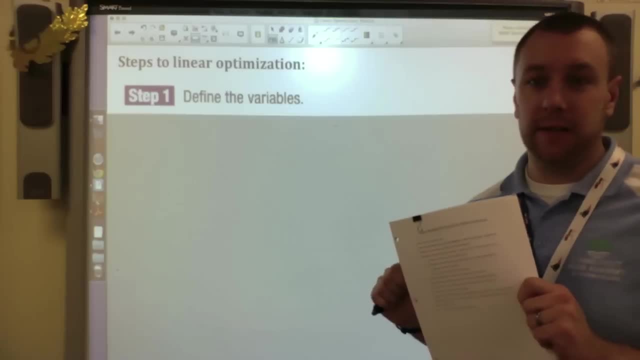 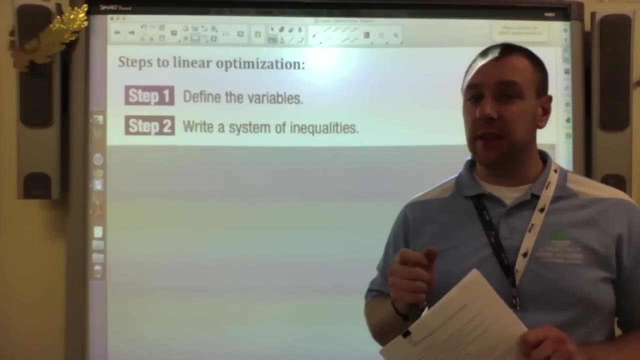 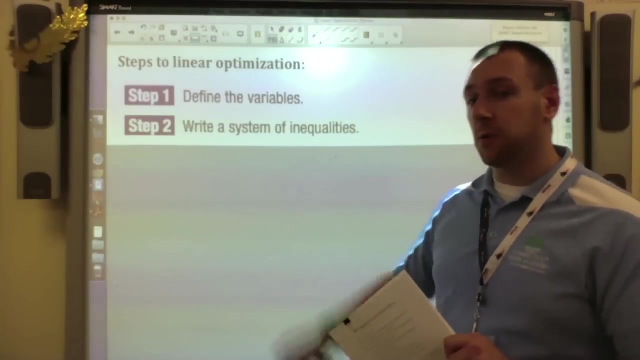 We're going to go through this process and it's going to help you define the variables. Step two: we're going to write a system of inequalities. okay, So that is the key. We've been practicing it for a while with equations. Now we're going to write some inequalities We're going to have. 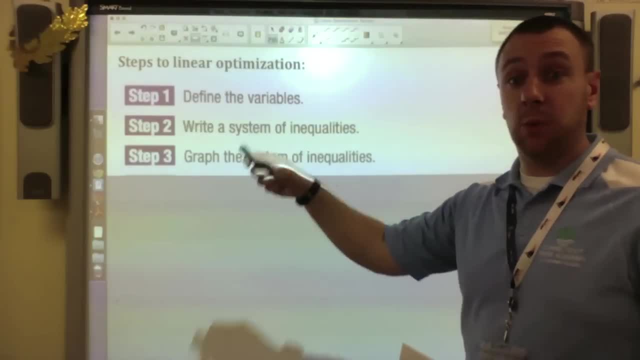 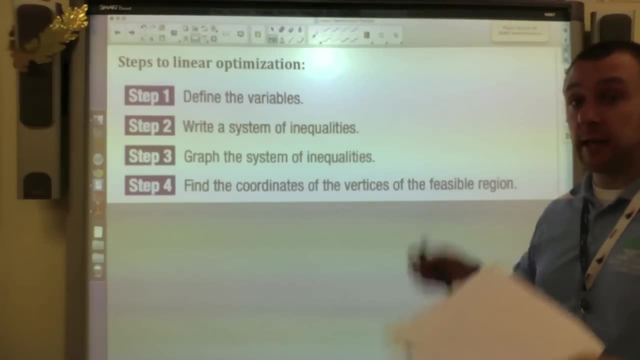 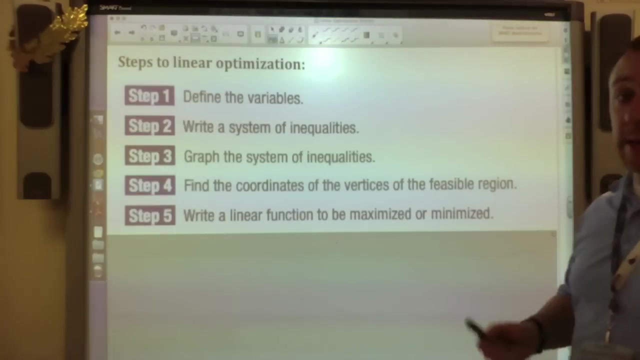 to graph the system of inequalities, just like tier one, okay, We then find the vertices. okay. So we find where it's shaded, okay, And we find the vertices for it. Then we write the linear function to be maximized or minimized. okay, This is what I'm calling the profit or the cost. 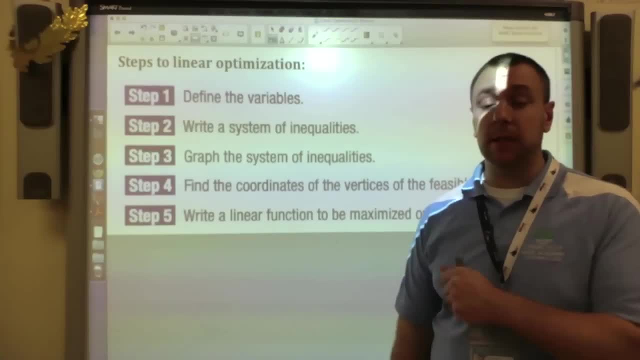 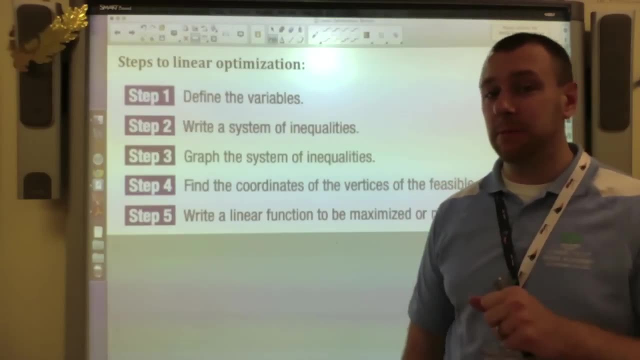 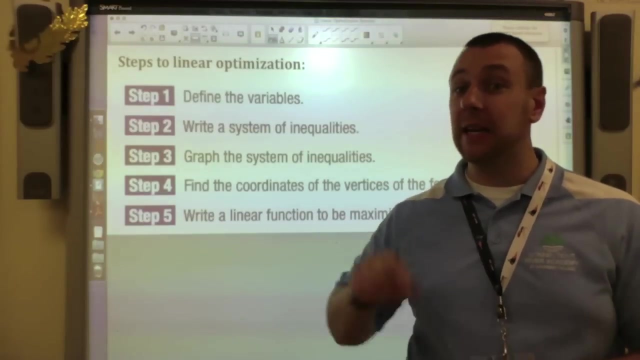 equation. Most times these are: we're trying to find the maximum profit that we have or the minimum cost. okay, So that's the biggest thing. It's profit or cost, And it's going to tell you what to maximize and what to minimize And that's going to be where you're. 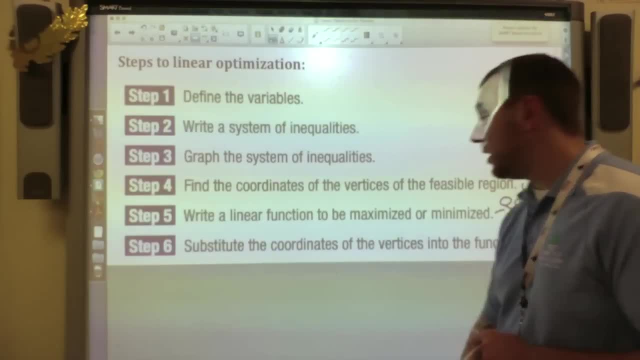 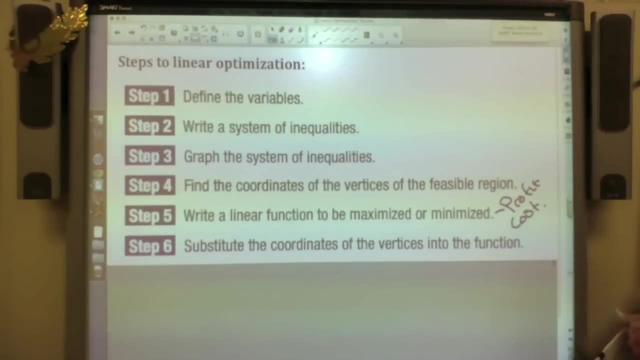 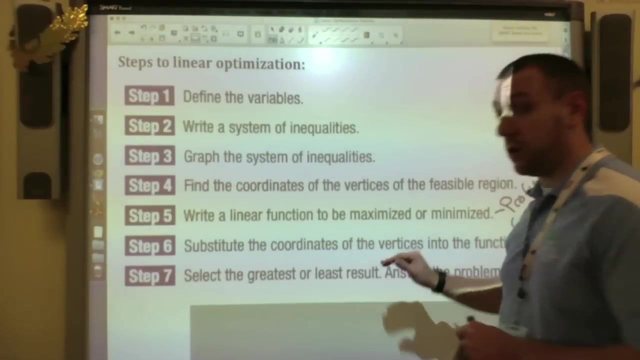 going to find the equation, Step six. again back to that tier one. We're going to take these vertices from step four and plug it back into that equation, And step six or step seven is to select the greatest or the least result. 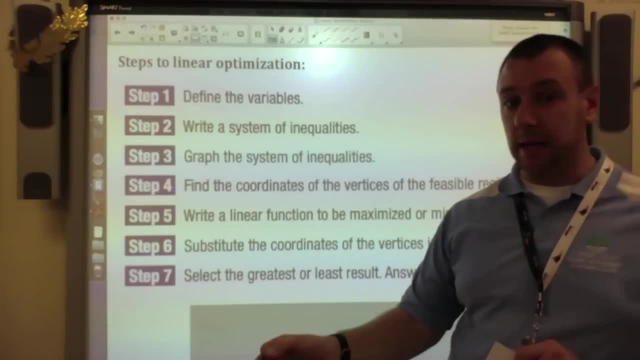 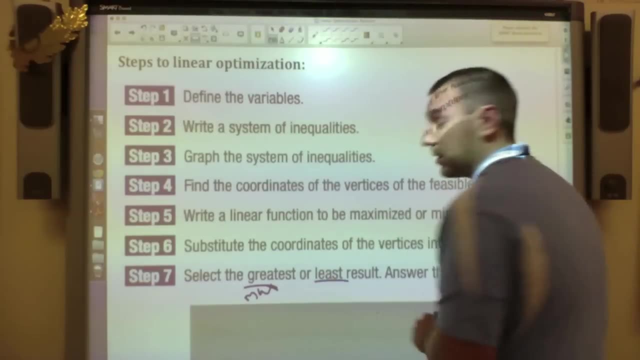 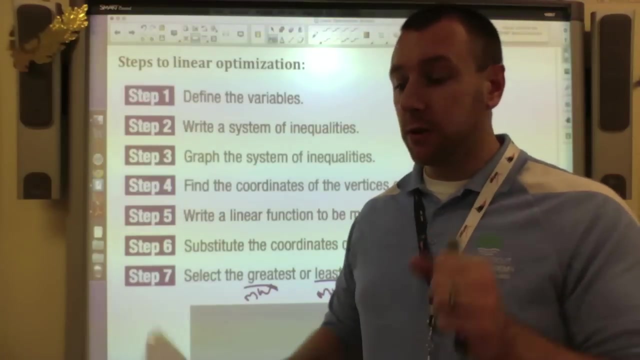 So that's the key. If it says to maximize, we're going to choose the greatest. We want the max. If it asks you to minimize, we're going to choose the least. Okay, So you have to make sure that you're answering the question. Okay, And that is part of our eight steps. All right, So let's go. 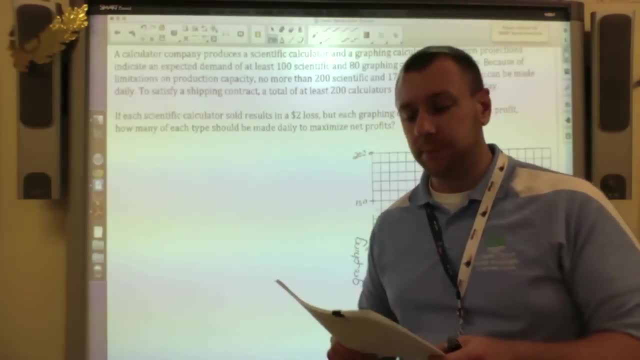 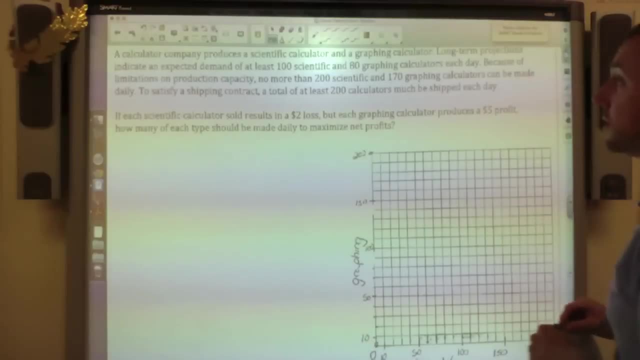 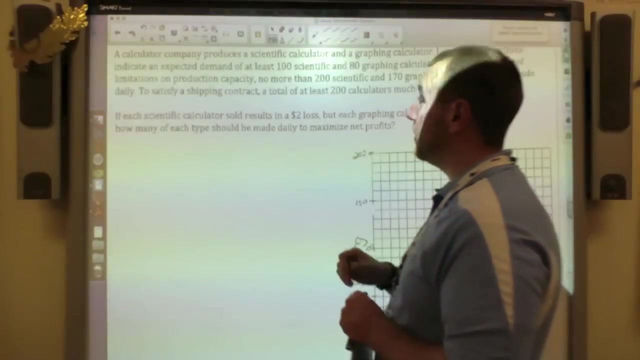 through this. Okay, And I'm going to follow this protocol. So the protocol tells me. I have to read the entire problem once. Easy enough. A calculator company produces a scientific calculator and a graphing calculator. The long-term projections indicate an expected demand of at least 100. 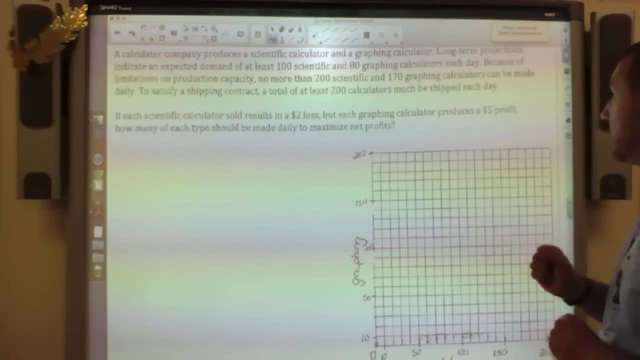 scientific calculators and 80 graphing calculators each day. Because limitations on production capacity, no more than 200 scientific and 170 graphing calculators can be made daily. To satisfy a shipping contract, a total of at least 200 calculators must be shipped each day. Each scientific calculator. 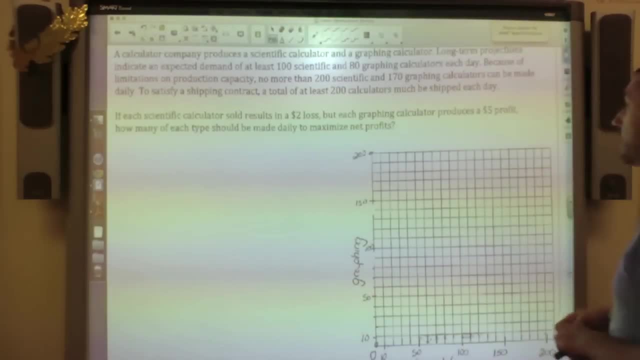 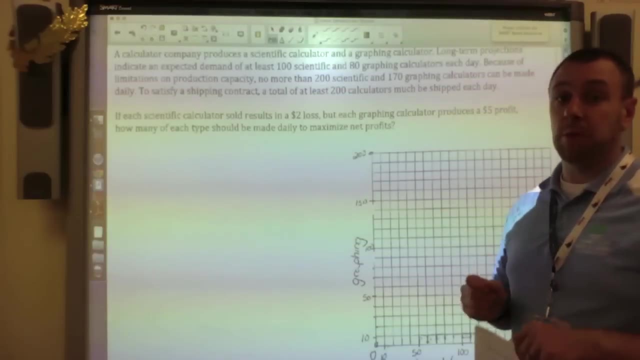 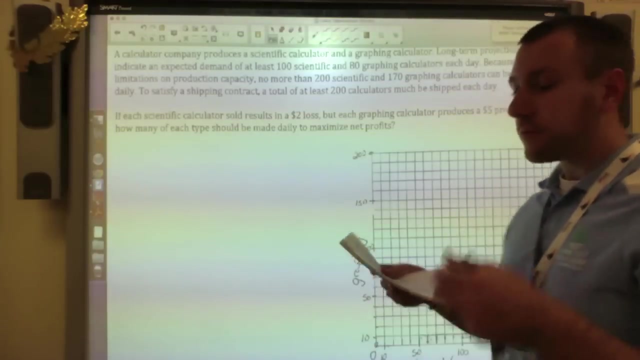 sold results in a $2 loss, but each graphing calculator produces a $5 profit. How many of each type should be made daily to maximize the net profits Done? I just read it. Okay, I'm not, I'm just reading it to understand. The second step is reread and identify what I'm trying to figure. 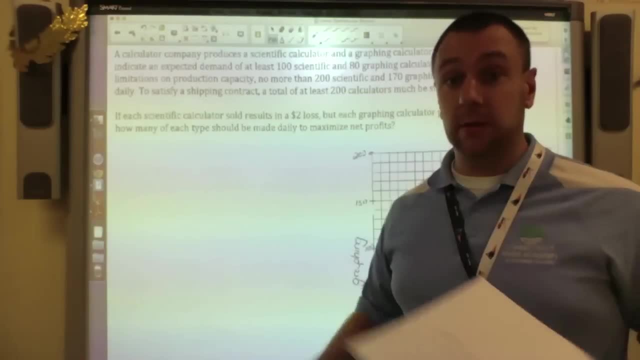 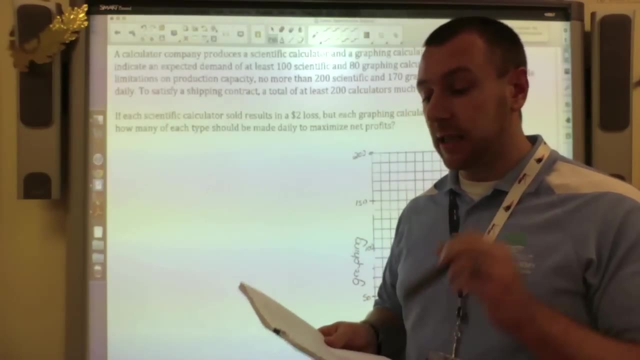 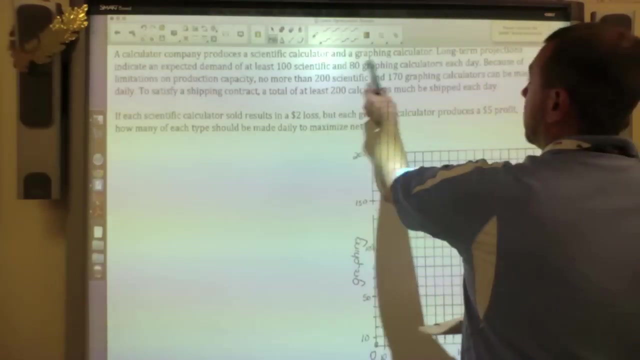 out. Okay, What is the problem or what it asking me to do? Okay, I'm not doing anything else, I'm just identifying. Okay. So calculator company produces a scientific calculator? Okay, There's no question there. Okay, Long-term projections indicate an expected demand of at least 100 scientific and. 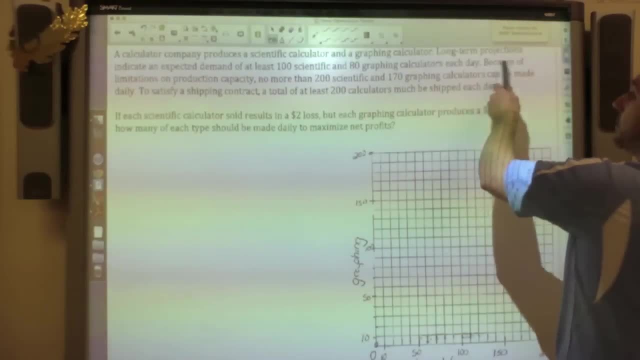 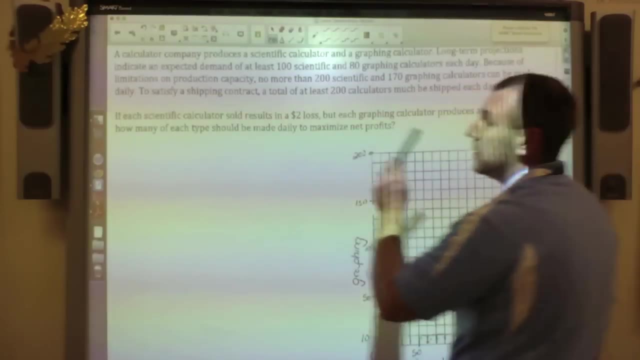 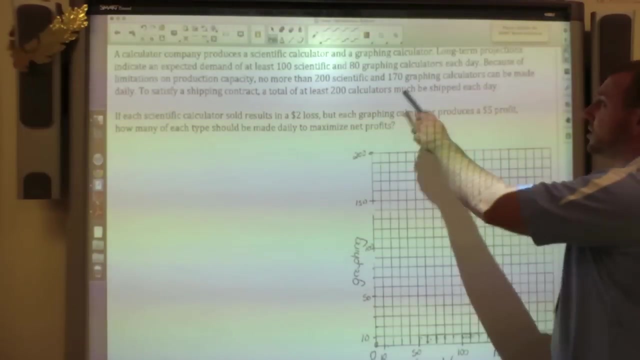 80 graphing calculators each day. No question there. Because of the limitations on production capacity, no more than 200 scientific and 170 graphing calculators can be made daily To satisfy a shipping contract. So there's no question there. Okay, These are just statements. Okay, If each 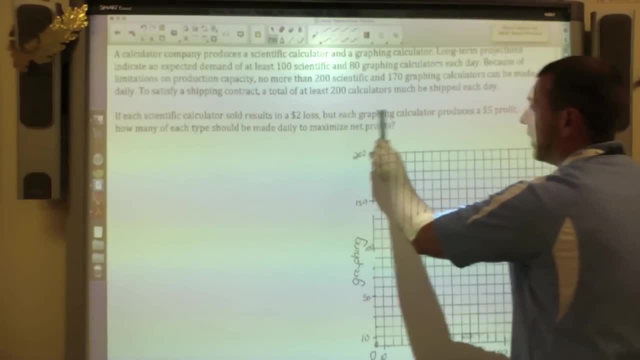 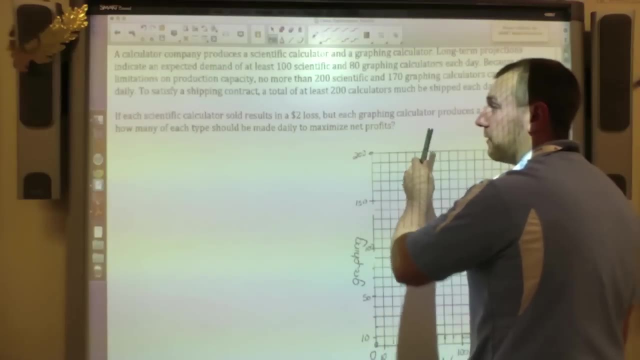 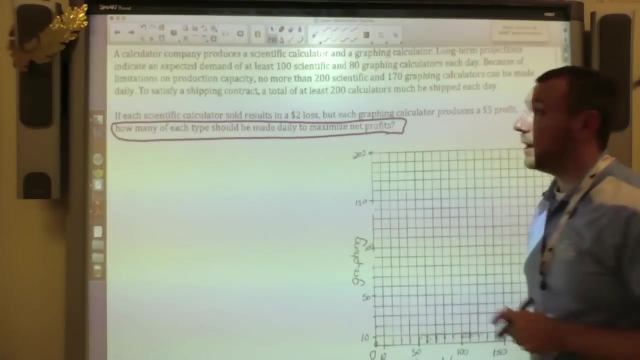 scientific calculator sold results in a $2 loss, but each graphing calculator produces a $5 profit. how many of each type should be made daily to maximize the net profits? This is where I find my question Okay, Number one key. you look for the question mark Okay, But not all things. 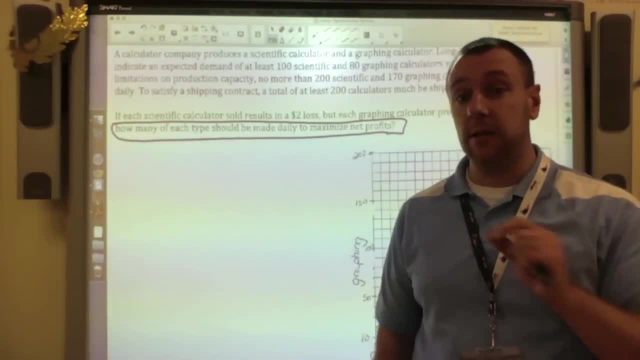 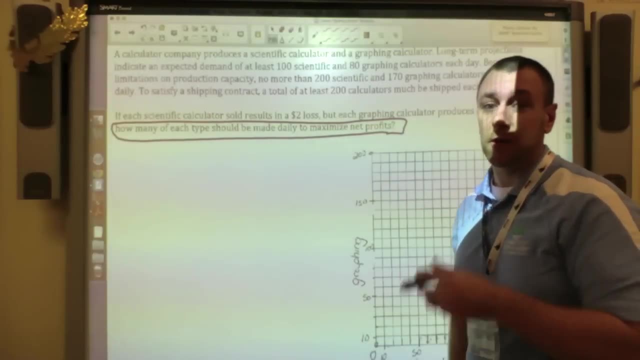 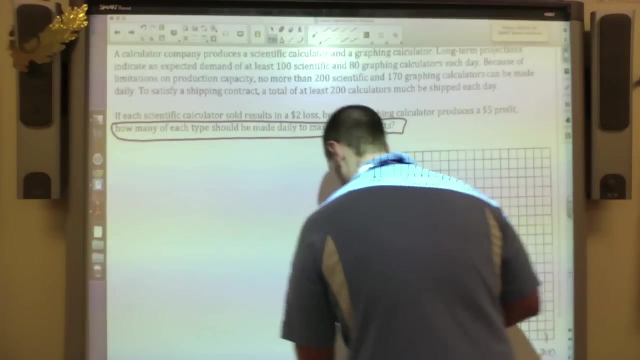 have a question mark. Sometimes they're statements like find, Okay, Or calculate. Those are statements, Sometimes they're not, with a question mark, So you got to watch what they're looking for, Okay, And what am I trying to figure out? How many of each kind? Okay, Each kind of what? Okay, And that's. 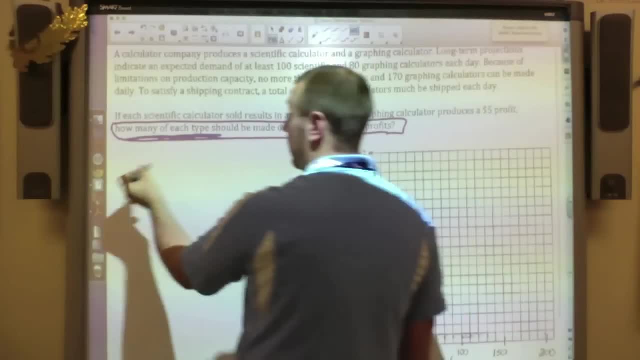 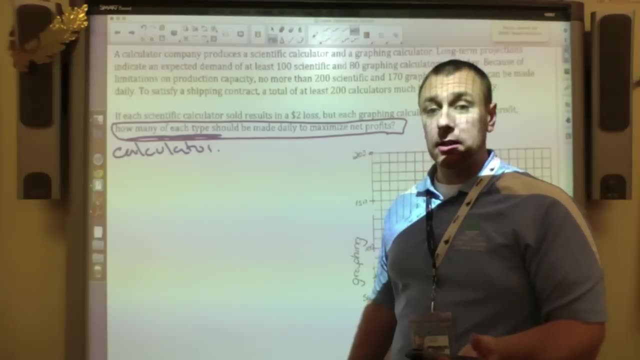 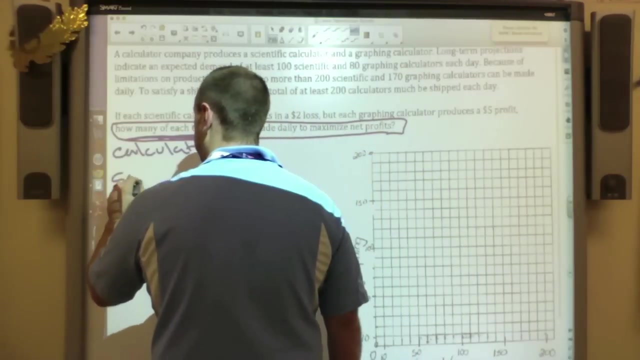 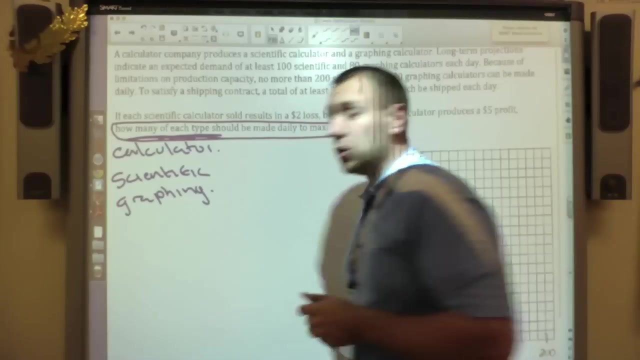 where I read the problem again. Each kind of calculator, All right, We're talking about calculators in this problem. That's the type of kind, Okay, And there's two types of kinds. Okay, There's the scientific And there's the graphing. Boom, Those are my two types And that's what it's. 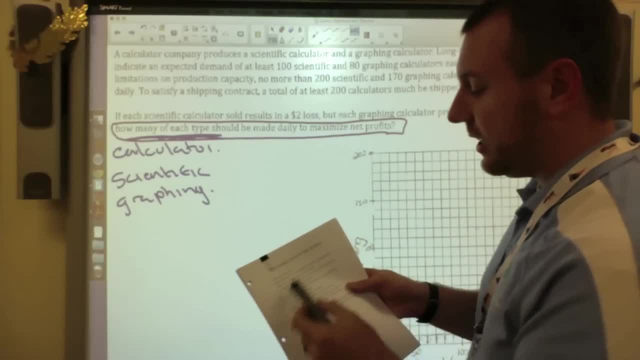 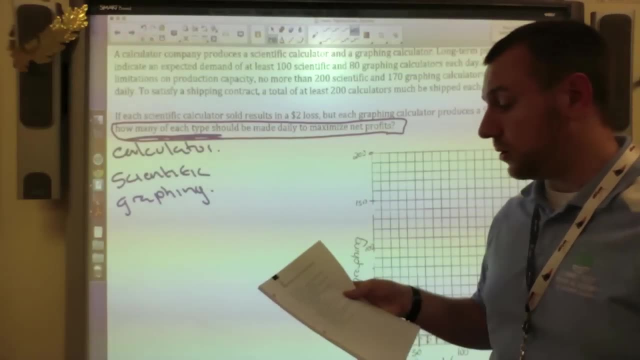 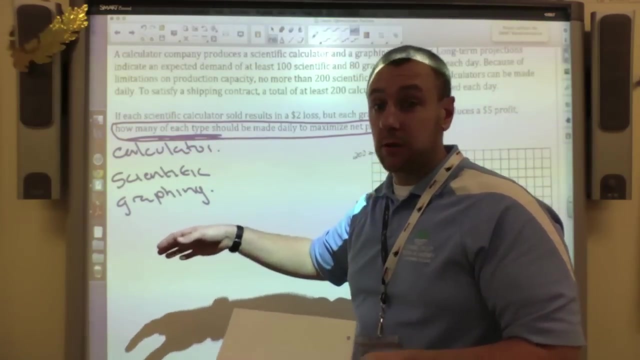 looking for Okay. Third step: Identify any unknown words or freezes. And you might know these, all these words, and some people don't. Okay, So the trick is, sometimes there's a lot of words in here that you don't know, Okay, Sometimes. 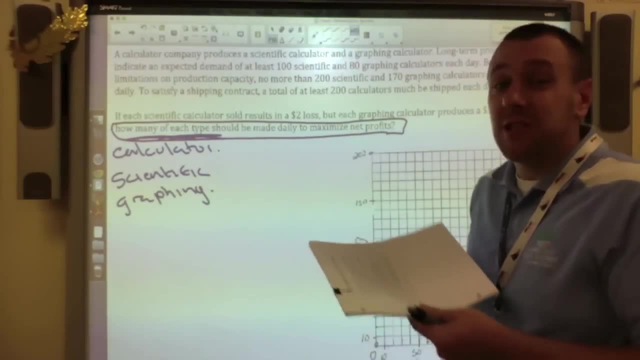 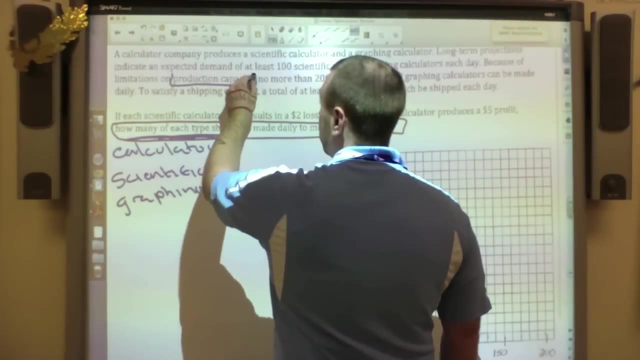 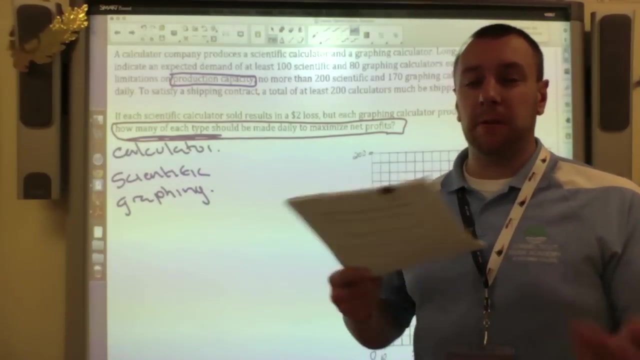 it's very simplistic And you just have to ask questions: Is this relevant, Is this not Okay? Some people might not know what production capacity? Okay, You just ask. Okay, You don't want to get caught up on vocab, Because a lot of times that's what holds people up. 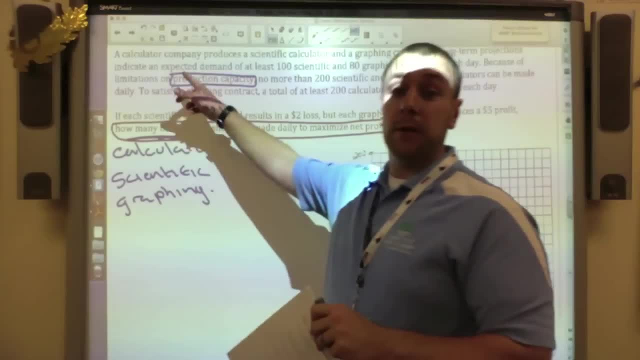 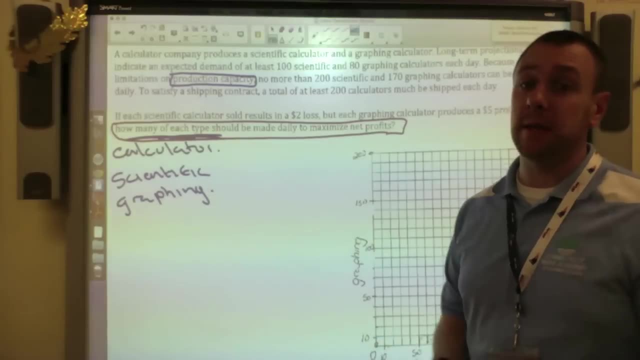 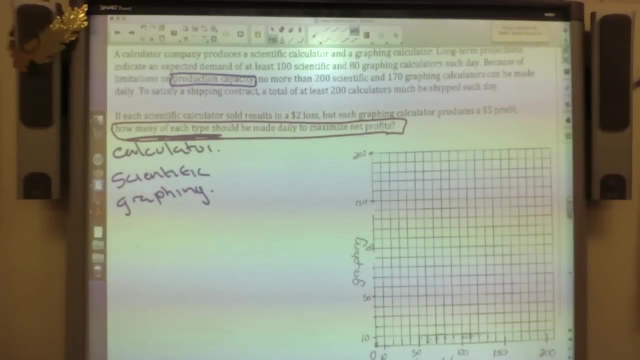 from word problems. Okay. So, by the way, production capacity is how much they can produce per day. Okay, They can't just do unlimited stuff, because there's a cap to what we can do. Okay, All right, So step four: Okay. 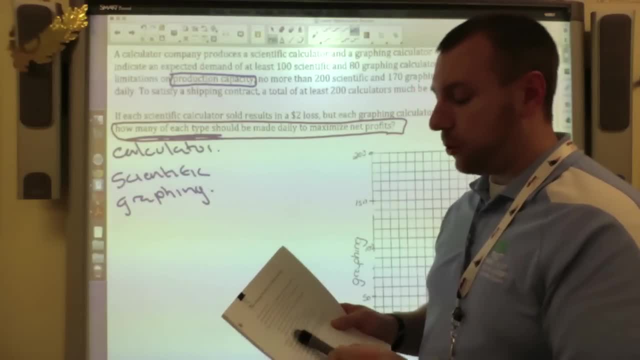 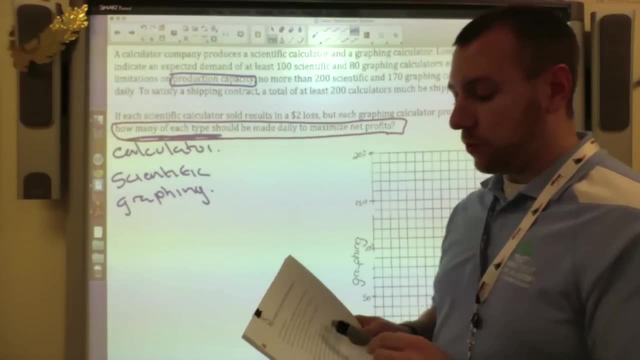 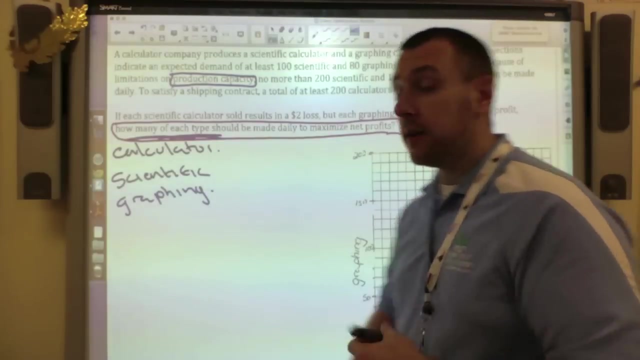 Has two parts: Identify the important information I need to be aware of- Okay. Part says: remove useless information in word problem sentences, All right. And part says: remove useless information from tables, charts or graphs. We don't have the table, chart or graph, But we can get rid of some useless him formation that. 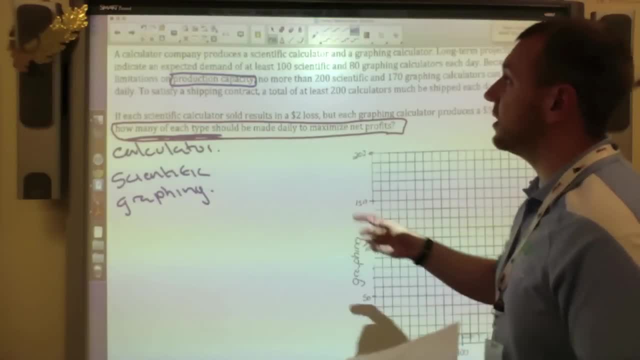 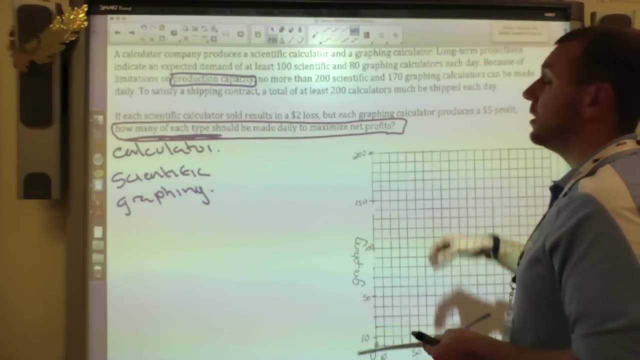 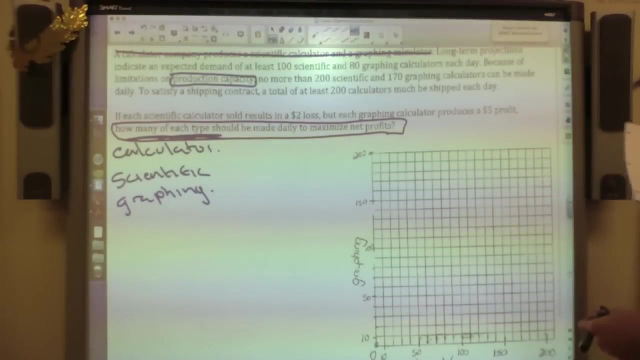 don't mean So. a calculator company produces a scientific calculator and a graphic calculator. Okay, but they talk about that after, so I don't need that sentence. Long-term projections indicate an expected demand of at least a hundred scientific and 80 graphing calculators each day. Do I care about? 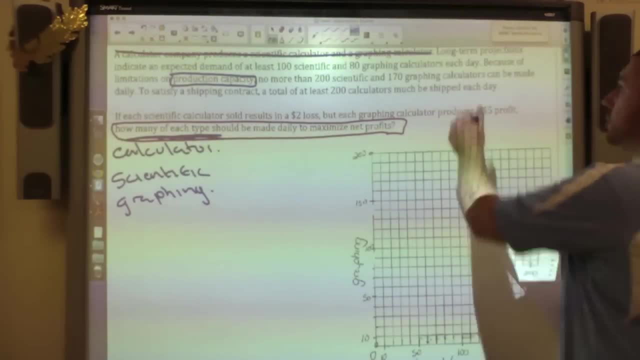 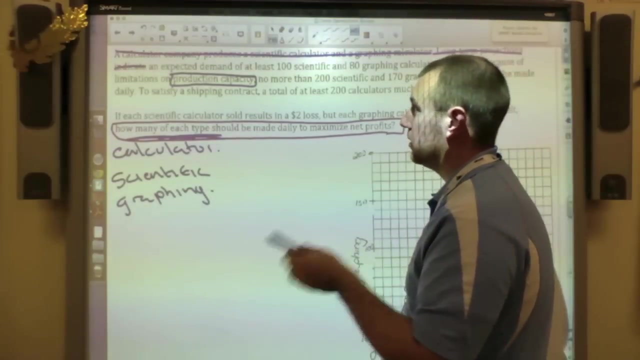 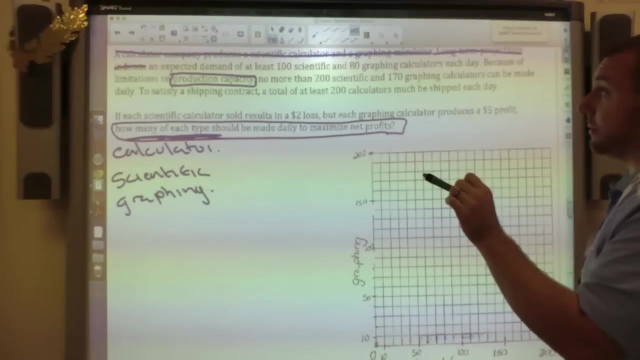 their long-term prediction. Okay, it just says that I have an expected demand of at least a hundred scientific and 80 graphing calculators each day. Because of limitations on production capacity, no more than 200 scientific and 170 graphing calculators can be made daily. 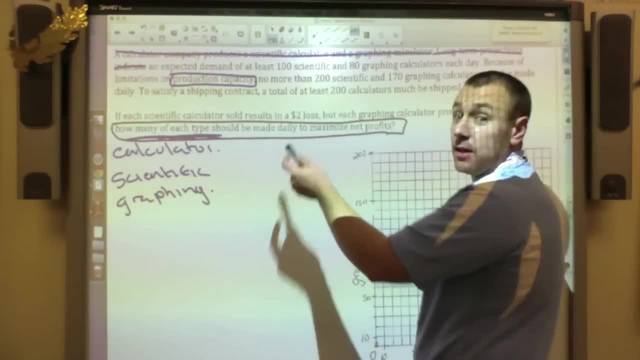 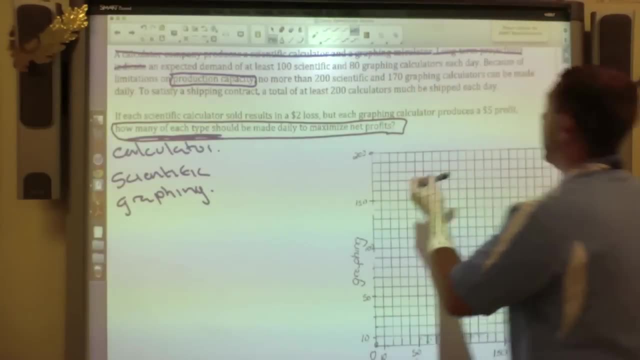 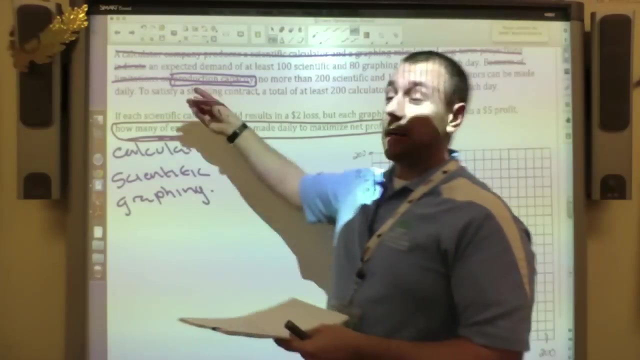 Well, really, it tells me that no more than 200 scientific and 170 graphing calculators can be made daily, So I don't even need to know that. So that word that I might have already known isn't even relevant, because no more than 200? Okay, I'm done. 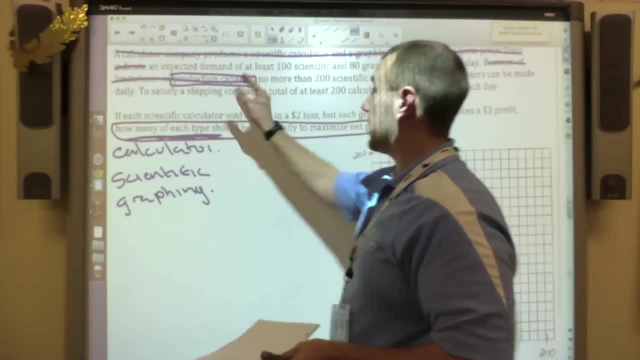 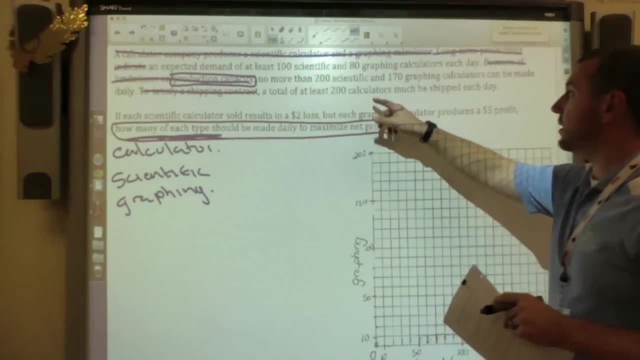 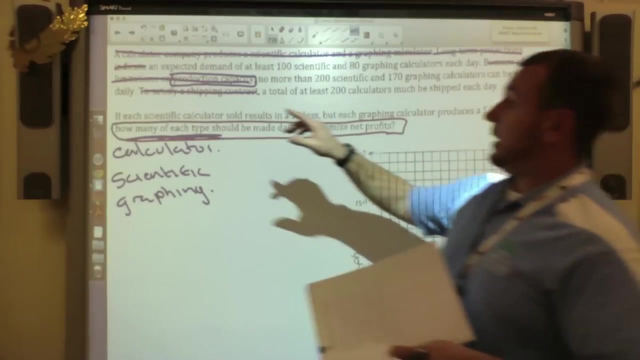 To satisfy a shipping contract. I don't care about the shipping contract. I don't care about the shipping contract. Okay, a total of at least 200 calculators must be sold, shipped each day. Okay, if each scientific calculator sold results in a $2 loss, okay, that's important. but 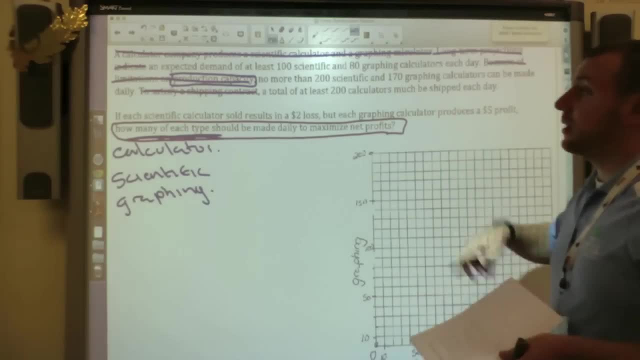 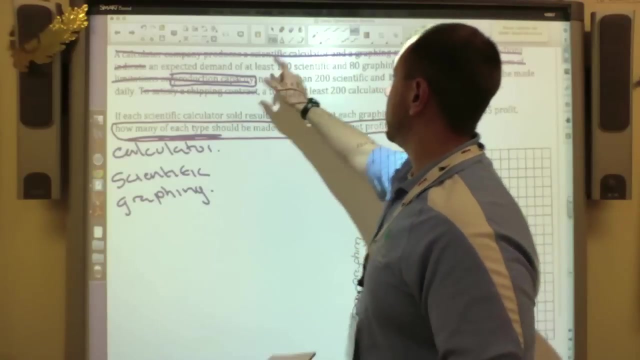 each graphing calculator produces a $5 profit. how many of each type should be made daily to maximize net profits? Okay, so that's all very important. Okay, so I'm just gonna reread this map wrong. Okay, an expected demand of at least 100. 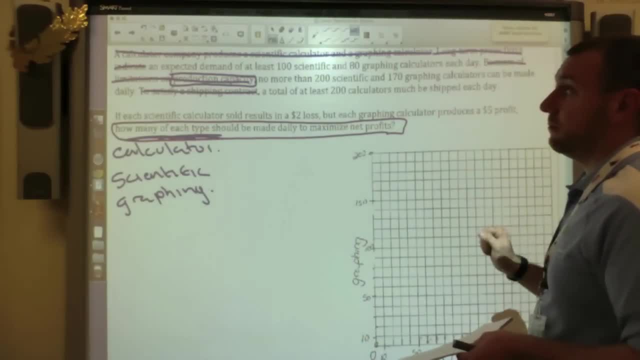 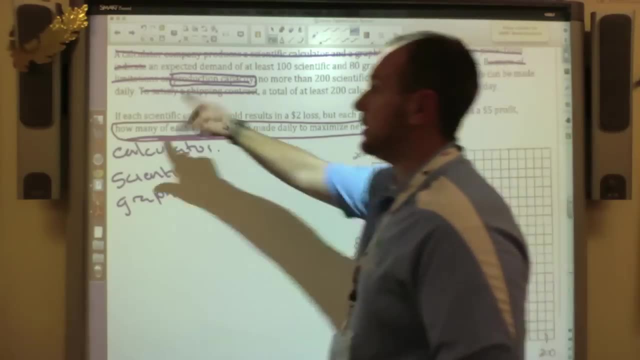 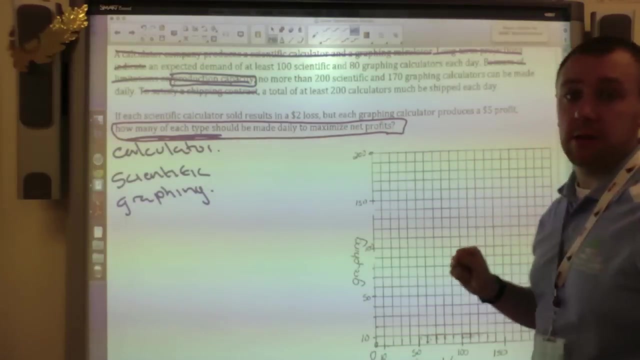 scientific and 80 graphing calculators each day. Okay- statement: we're good. No more than 200 scientific and 170 graphing calculators can be made daily. Statement: we're good. A total of at least 200 calculators must be shipped each day. 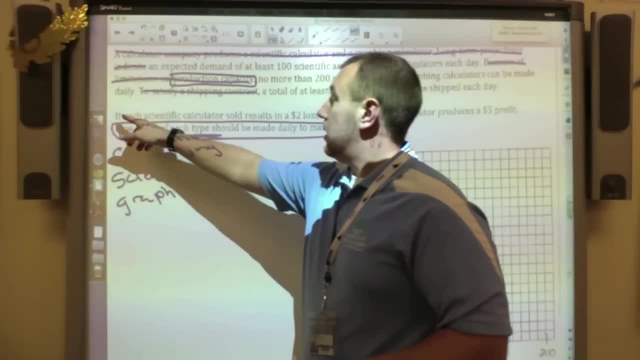 Statement good. Okay, if each scientific calculator sold results in a $2 loss, but each graphing calculator must be shipped each day. Okay, if each scientific calculator sold results in a $2 loss, but each graphing calculator produces a $5 profit. how many of each type should be made daily? 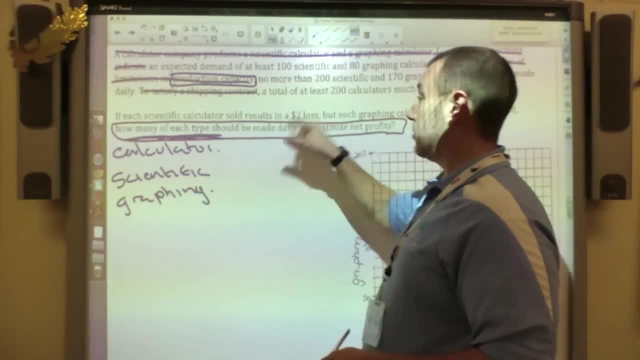 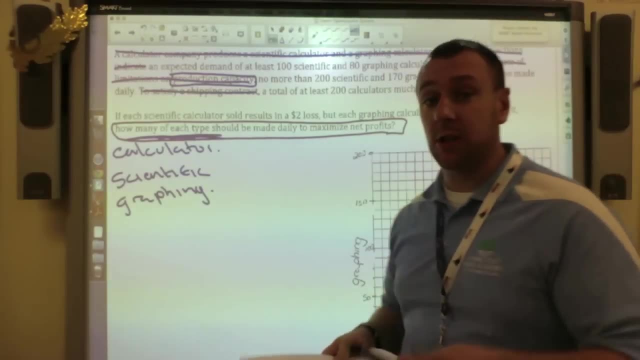 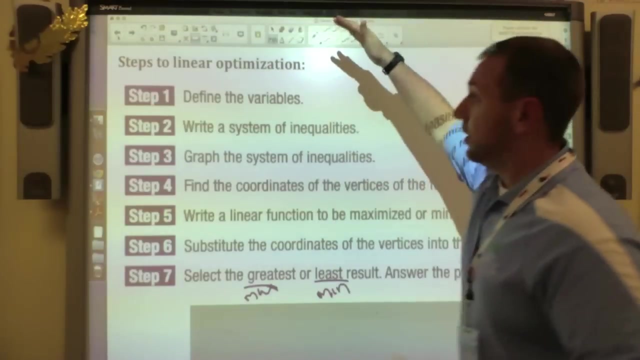 produces a $5 profit, How many of each type should be made daily to maximize net profits? Okay, so now we have to classify the problem and identify the procedure we're going to solve. We already know this is a linear optimization problem and the procedure here is right here. Okay, so now. 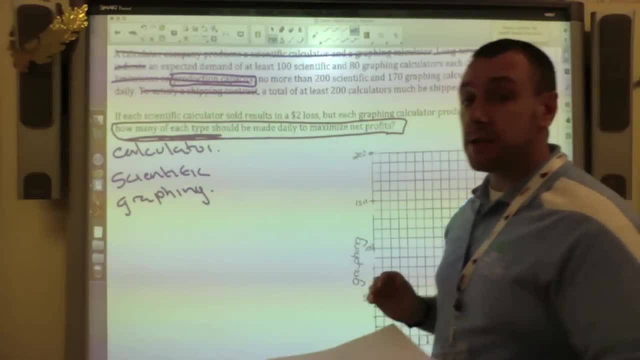 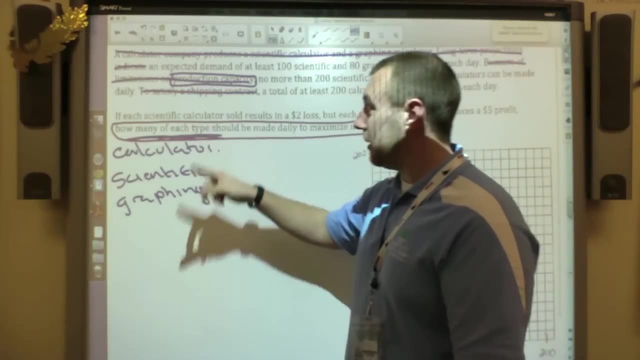 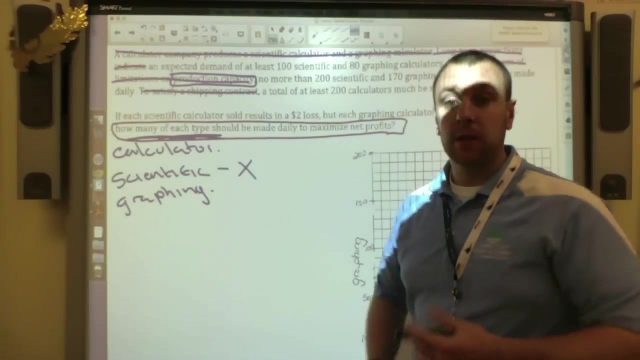 we're going to go through those steps. Okay, the first step is to define the variables. Well, we're talking about two things, right- right here- how many each type? Well, we're talking about calculators. There's two types: Scientific, I'm going to call that X. Grappling, I'm going to call Y. Okay, Boom. 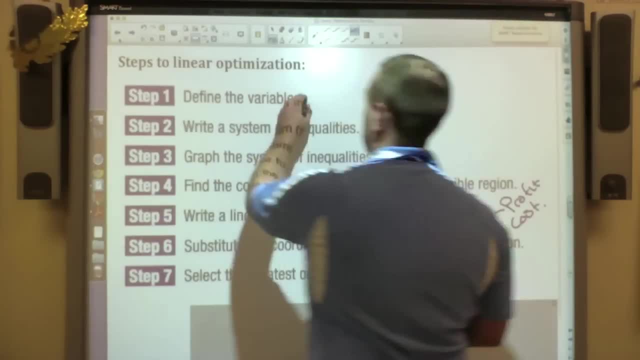 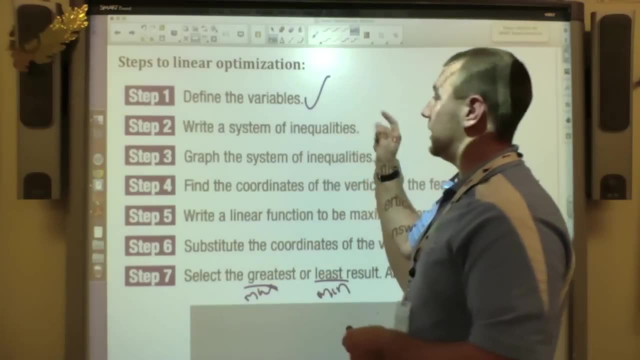 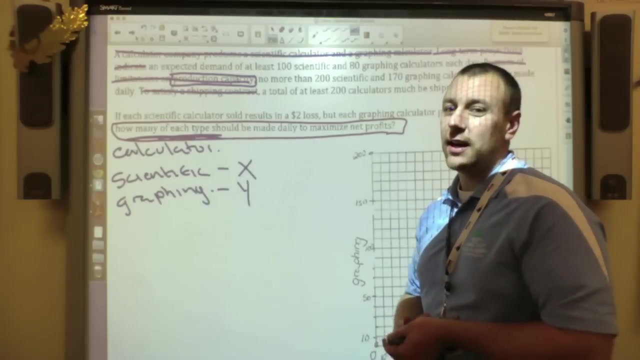 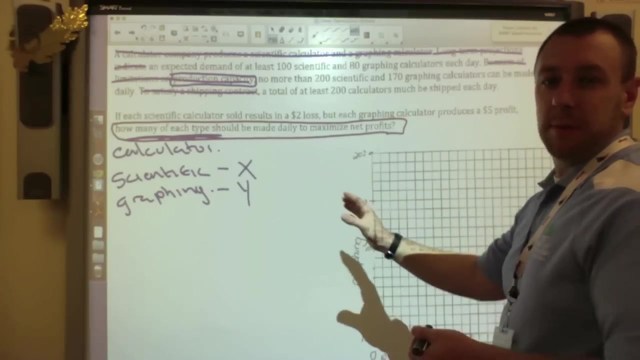 Done, All right. So check, I defined it: X is scientific, Y is graphing. All right- write a system of inequalities: Well for linear optimization- Well for linear optimization- Well for linear optimization- there's always two easy ones: okay, X okay. we're never dealing with negative. people can't do. 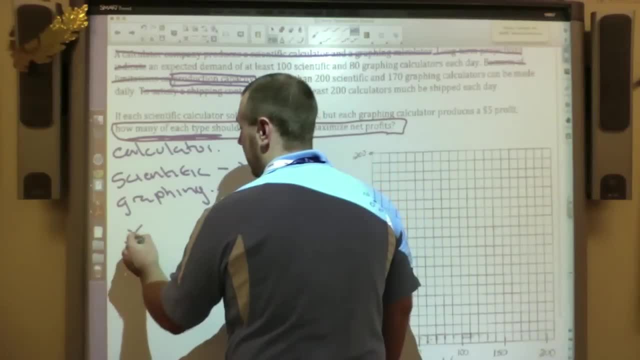 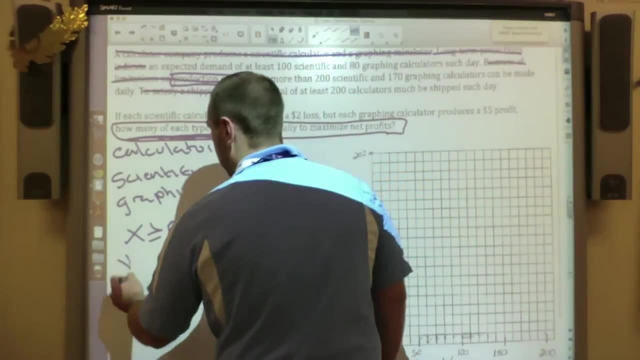 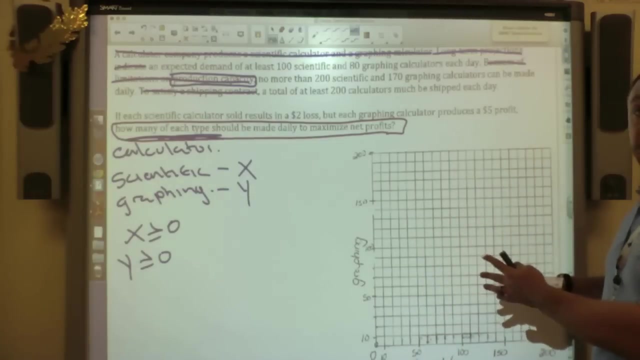 negative stuff, right? so X has to be greater than or equal to zero, because we got to produce some scientific stuff, and Y has to be greater than or equal to zero. we're dealing with something that's positive, right? so if you get a negative result, you did something wrong, okay, so now we 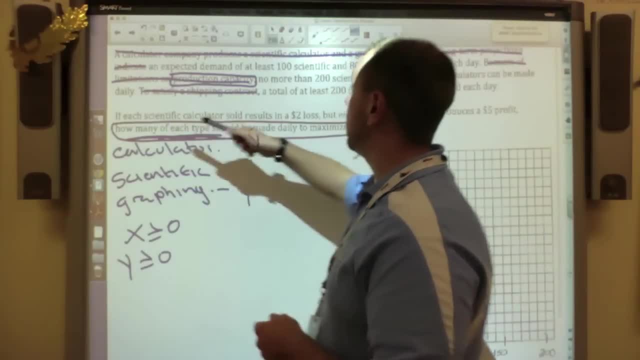 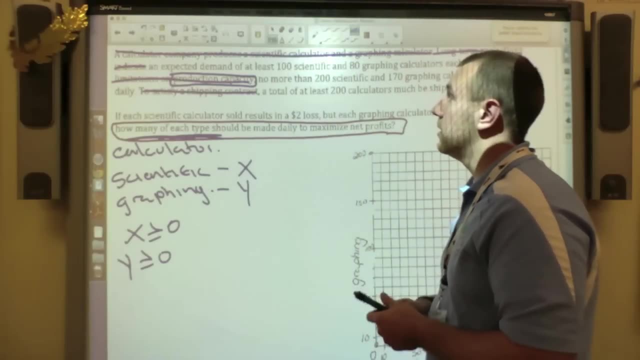 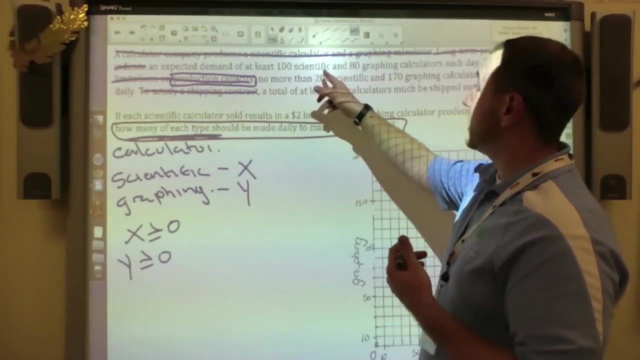 read the sentences again: an expected demand of at least a hundred scientific. expected the man- of at least a hundred scientific. okay, scientific, every time you see that word X. okay, so X has to be at least a hundred. so X has to be greater than or equal to zero, because we got to produce something. 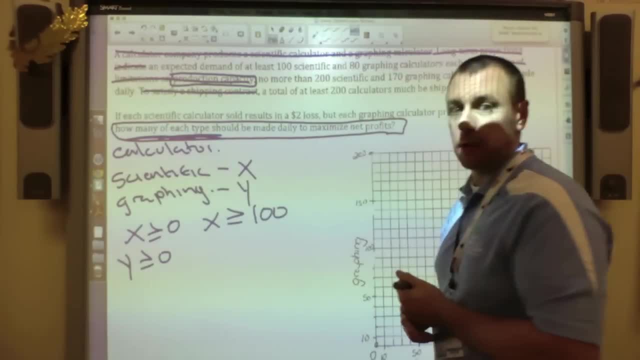 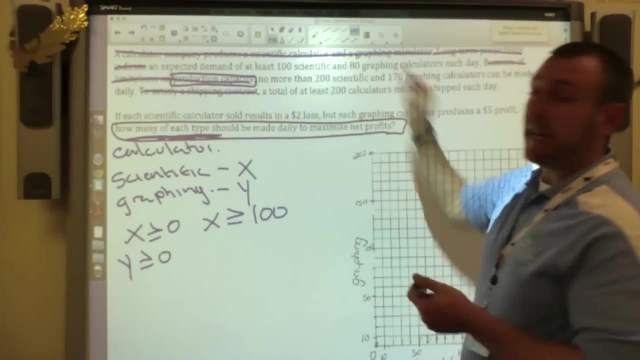 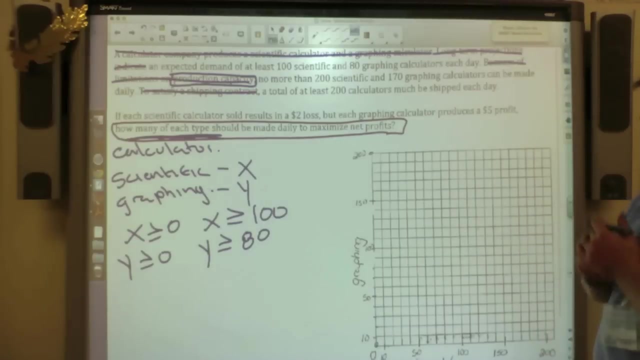 or equal to 100, all right, and 80 graphing calculators each day, So graphing calculators has to be at least 80.. So y has to be greater than or equal to 80.. All right, I got that information. 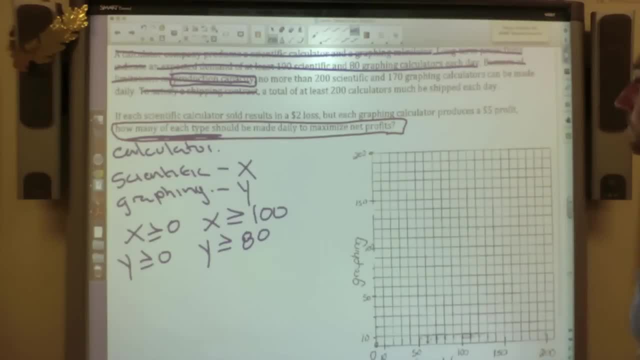 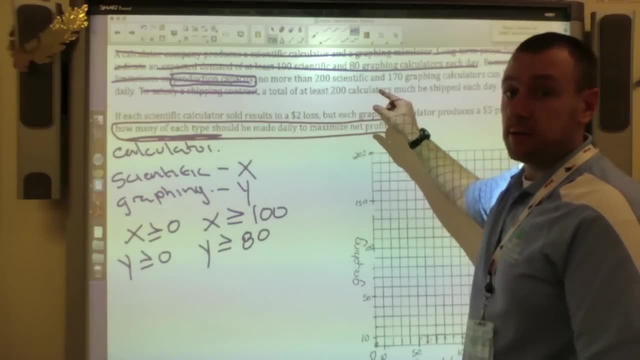 Now I'm going to kind of cross that out, I don't want to go back to it. All right, no more than 200. scientific, No more than 200.. Okay, so I can produce at least 100, but I can't go over 200. 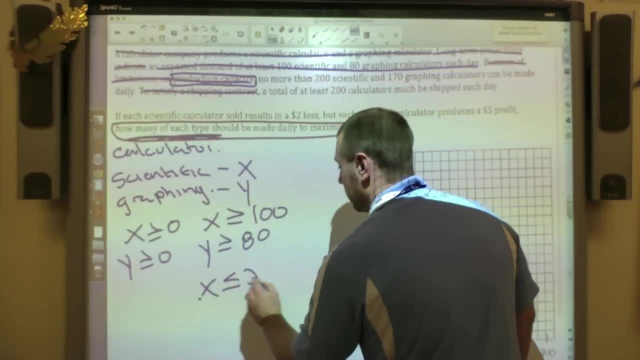 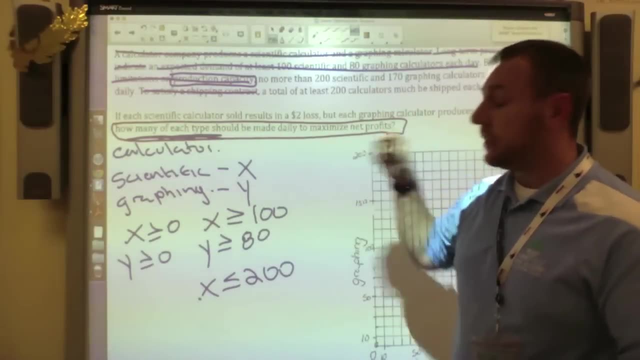 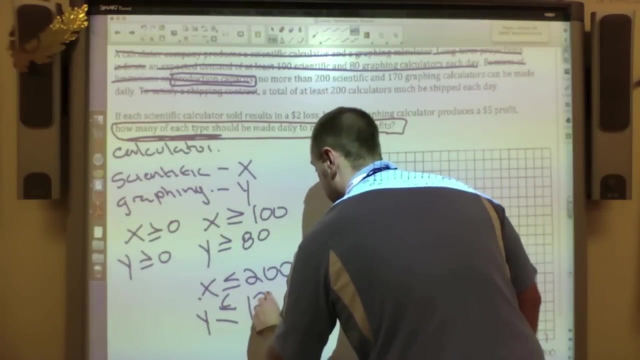 So x has to be less than or equal to 200.. All right, and 170 graphing calculators can be made daily. So that's my cap, That's my max. So y has to be less than or equal to 170.. All right, 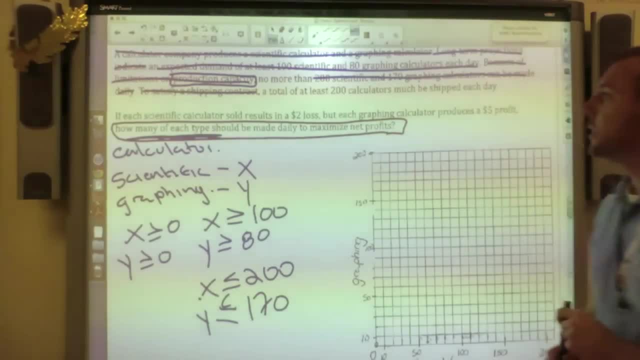 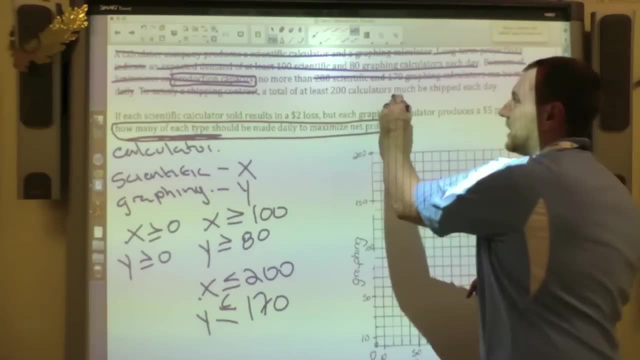 now, I got that information, Got that information down. Okay, at least a total of at least 200 calculators must be shipped each day. Calculators- Well, I have two different types, right, I have my scientific and my graphing. 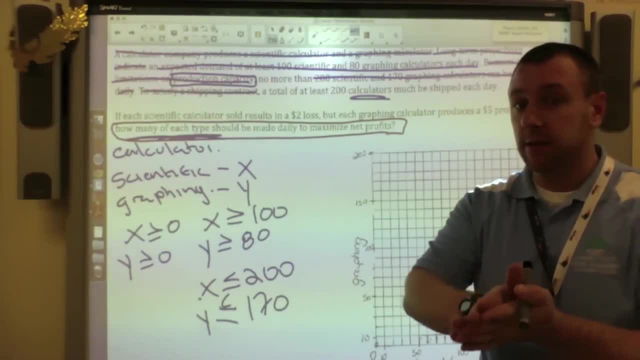 So when I combine them, when I put them together, they can't go. they have to be over 200, right? So when I combine them, every time we combine something in math it's just addition. So I'm going to take my scientific. 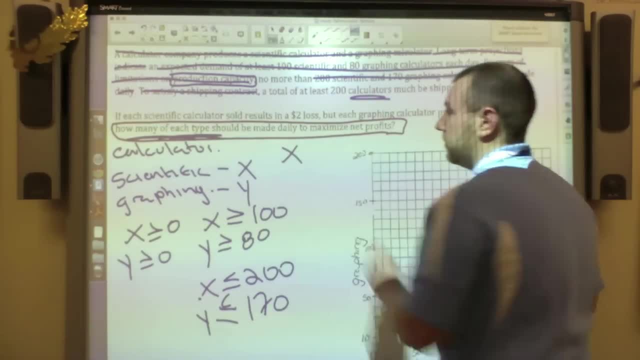 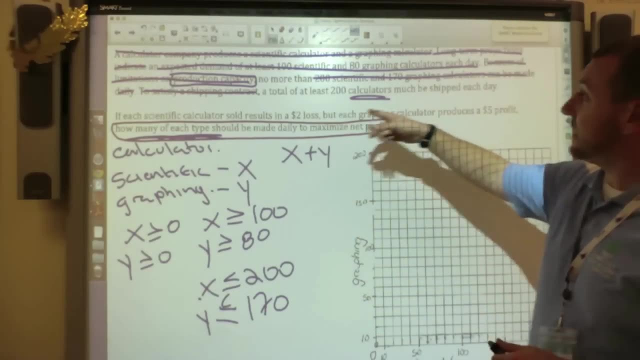 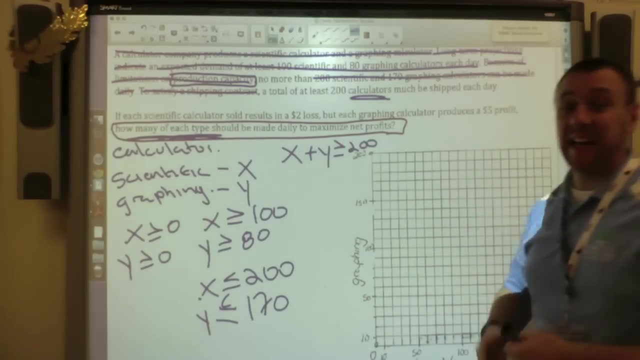 My x And I'm going to take my graphing y and I'm going to add them together And I have to get at least 200.. So this has to be greater than or equal to 200.. I got awesome inequalities. now, Okay. 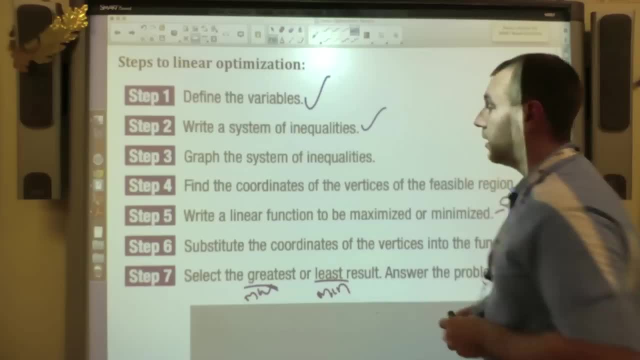 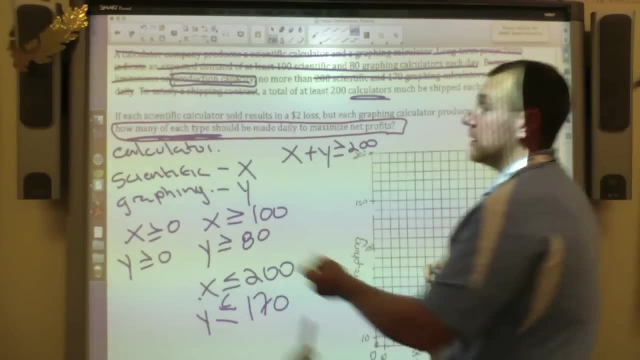 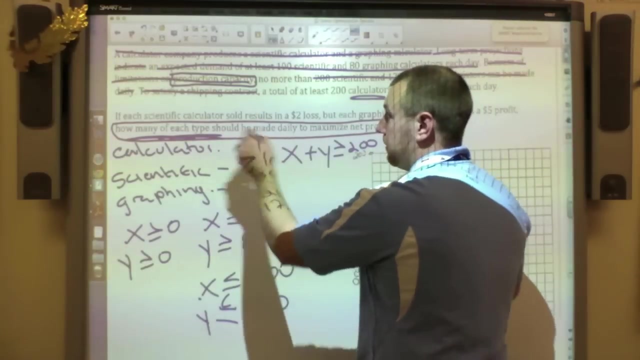 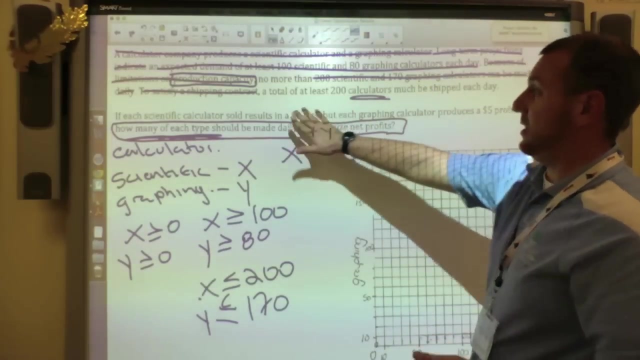 Okay, Boom, I'm going to graph the system of inequalities. Okay, Well, actually, let's go back to this. If a scientific calculator results in a $2 loss, but each graphing calculator produces a $5 profit, how do I maximize it? Well, is there anything that's equal to No? So that is. 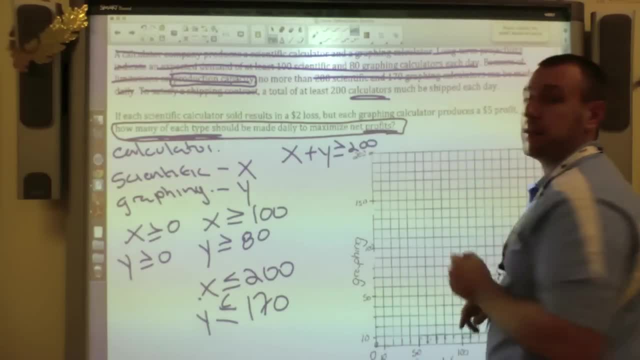 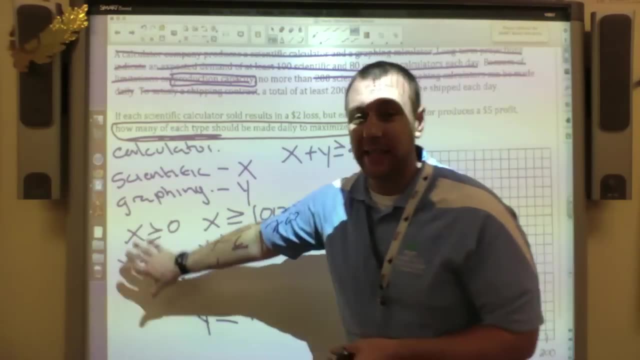 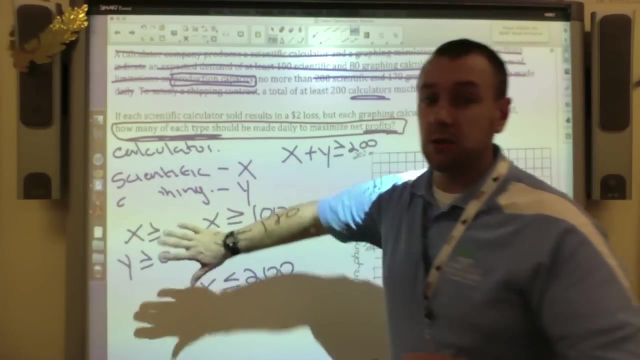 going to be a separate thing. That is going to be my graphing equation later. All right, So I'm going to graph all of these. These equations here make these irrelevant. Okay, Those are more of the things that I can always start with, So you can ignore those. right now I'm just going to graph. 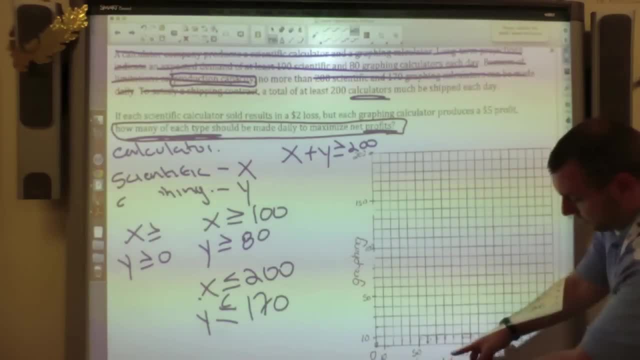 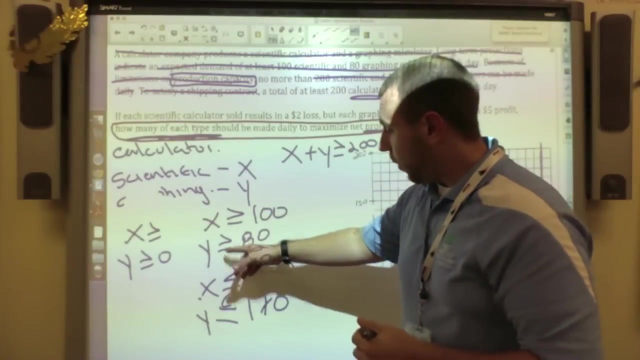 these. Well, vertical, vertical. So I know my scientific over here is 100 vertical, Okay, But it's got to be less than 200 here, Okay, And somewhere in between these, All right, Y has to be between 80 and 170.. So 60, 70, 80. Okay, It has to be between 80 and 170.. So I'm going to graph. 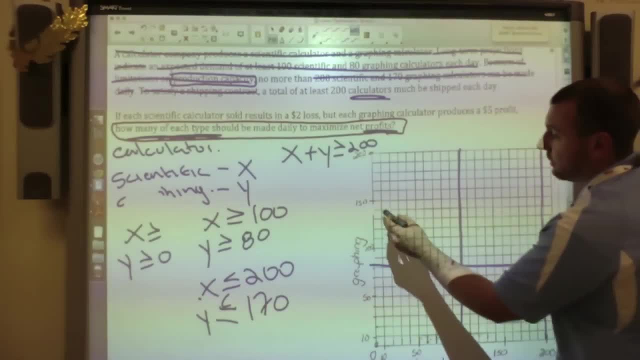 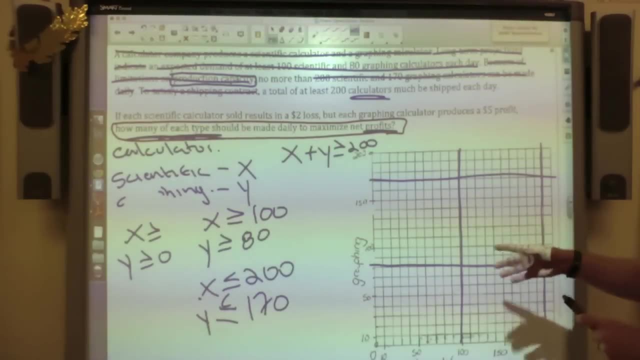 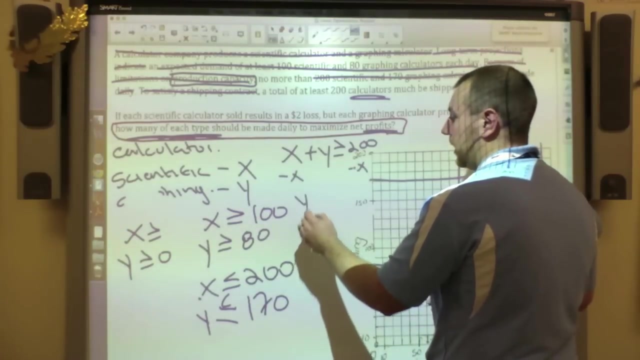 it. It has to be here to 170, here, Okay. So it's somewhere in here. Okay. So now I have to graph this part. Well, I have to solve for y. So y is greater than or equal to negative x plus 200.. 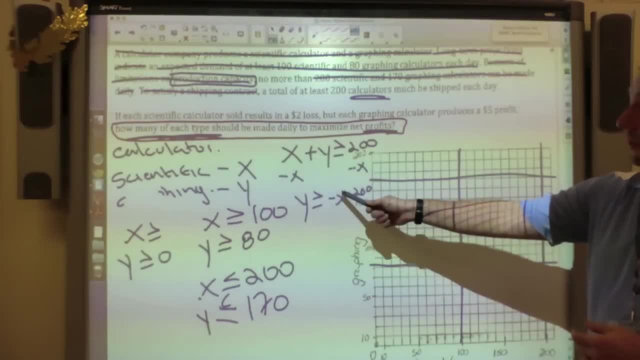 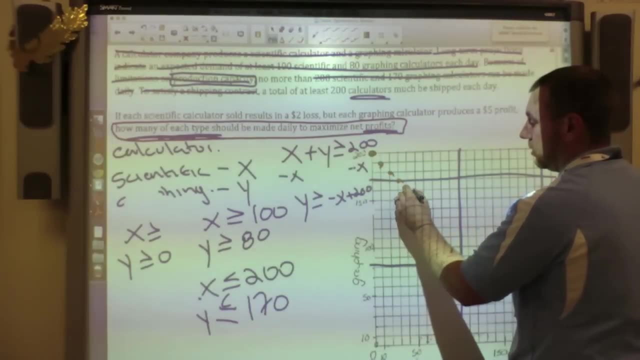 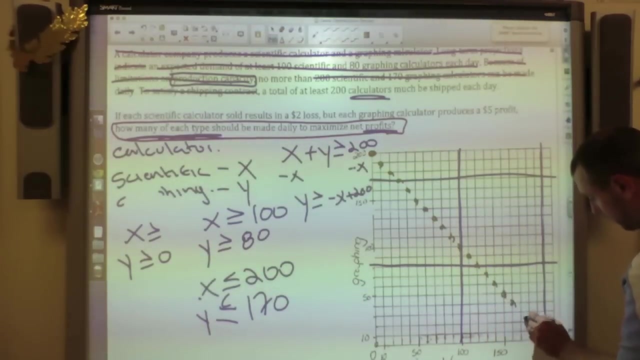 Okay. Well, back to my b. My slope is negative 1.. So I'm going to plot, Okay, And I'm just going to continue some points down. So I know, Okay, And it's going to be like that. 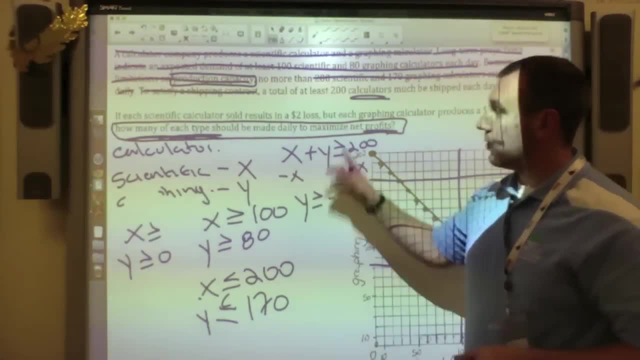 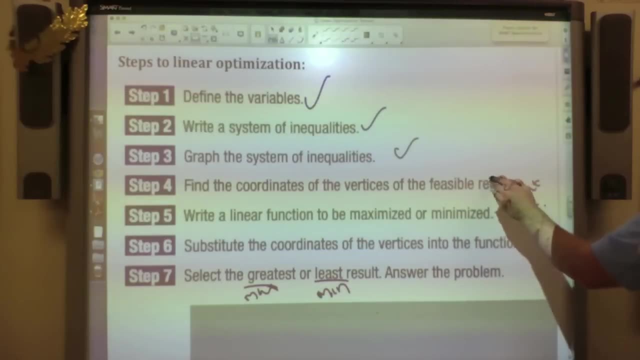 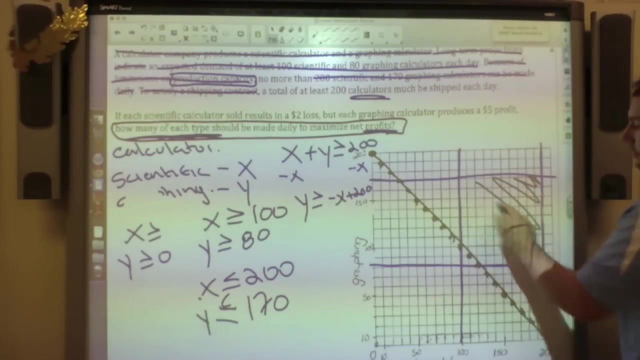 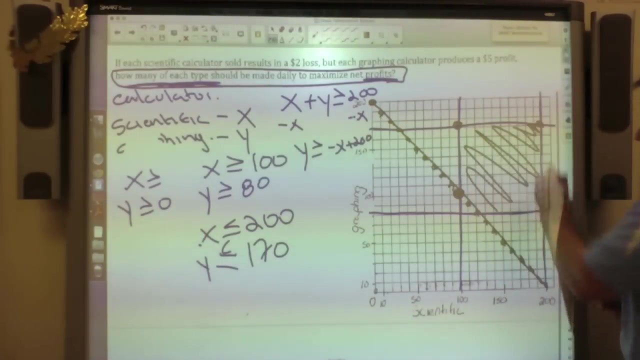 Okay. So now, okay, I've graphed it. Okay, Check. Find the vertices for the feasible region. Okay, The feasible region's in here, Because it's got to be greater than this and in between all this stuff. Okay, So all I'm going to do is find the vertices. All right, So they're here, here, here. 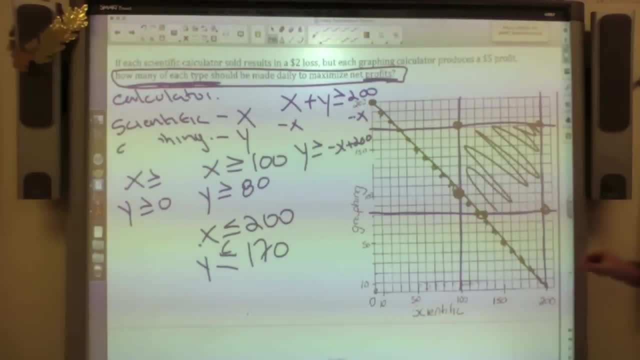 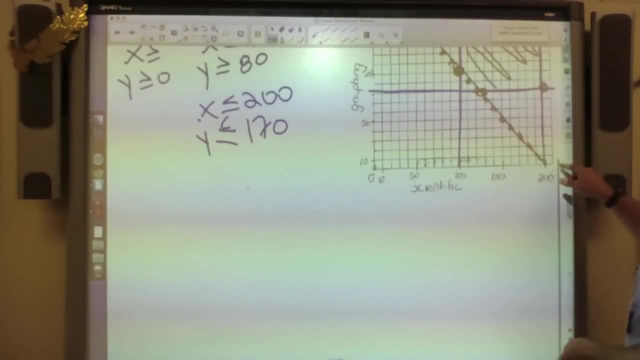 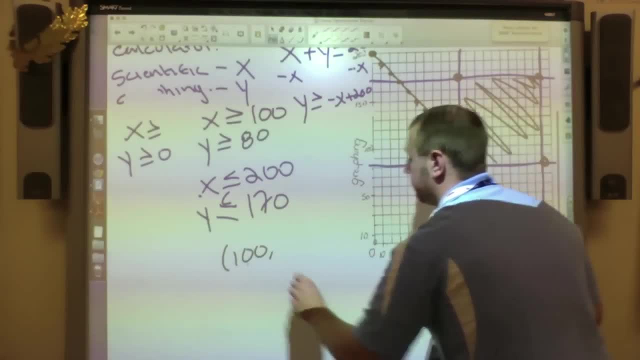 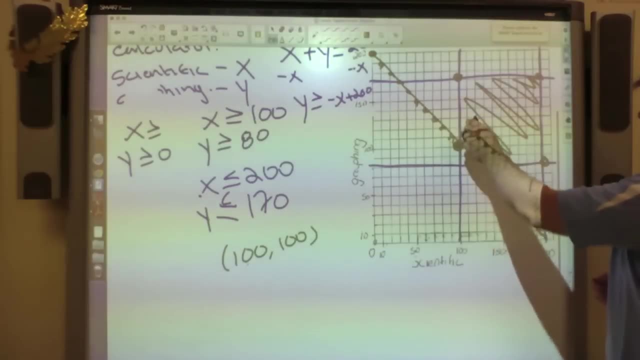 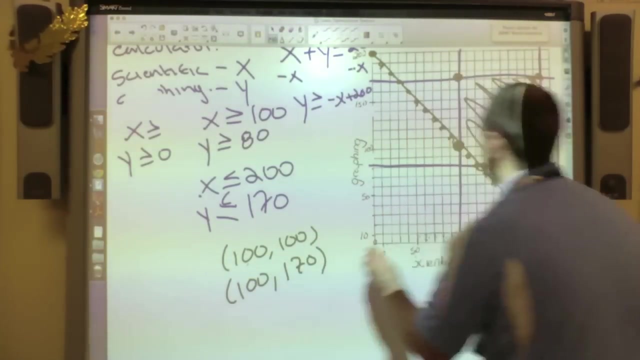 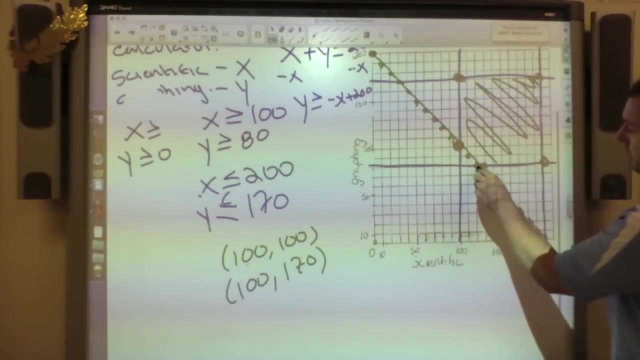 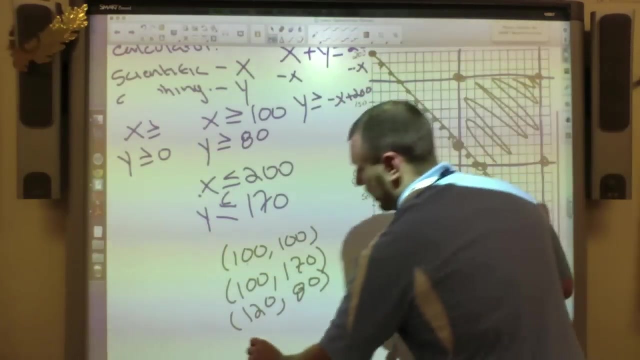 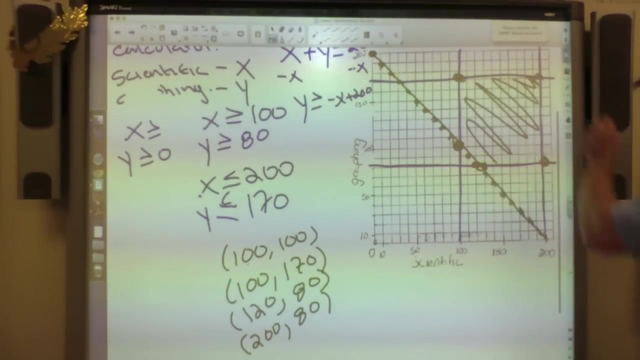 Okay, 100 goes to the x. Right, 100.. Okay, 100.. 170.. This point right here. Okay, I then have 120.. and 80.. I then have 200 and 80, and I have 200 and 170.. Okay, So that's my feasible region. 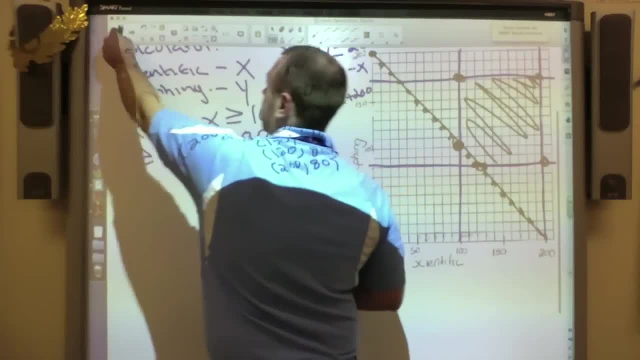 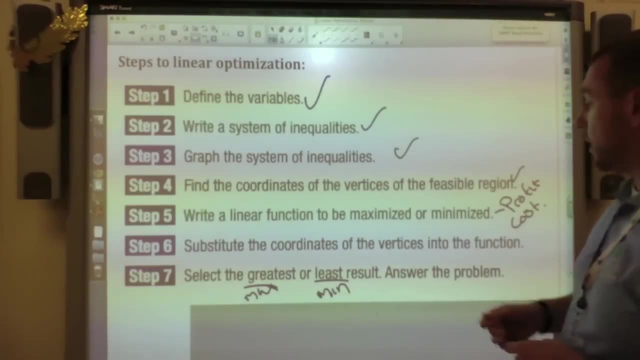 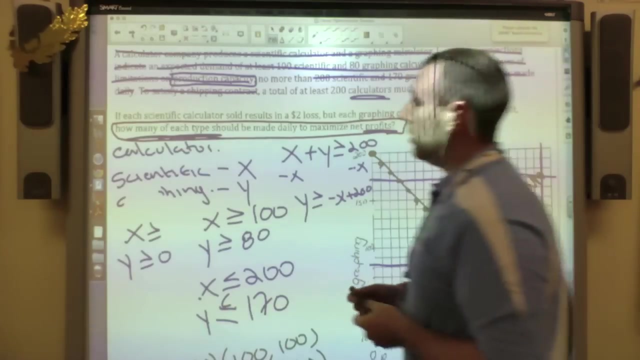 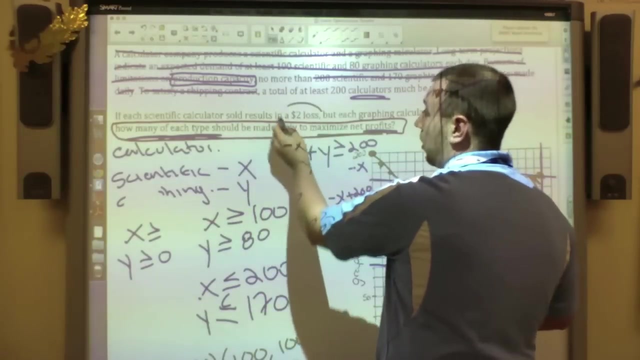 Okay, Those are my vertices. Check. Now I have to write a linear function to be maximized or minimized. Okay, So they use these words in here and they also use profit and cost. So how do I maximize that profit? Well, scientific calculators sold results in a $2 loss. 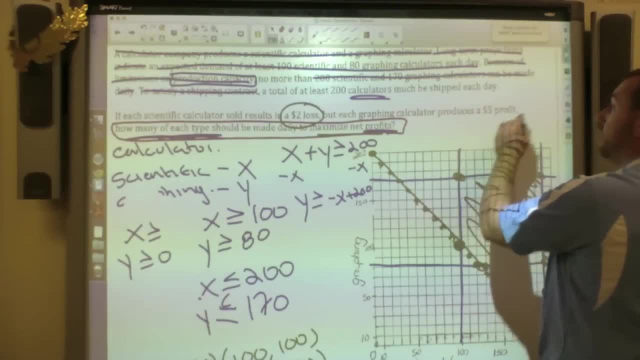 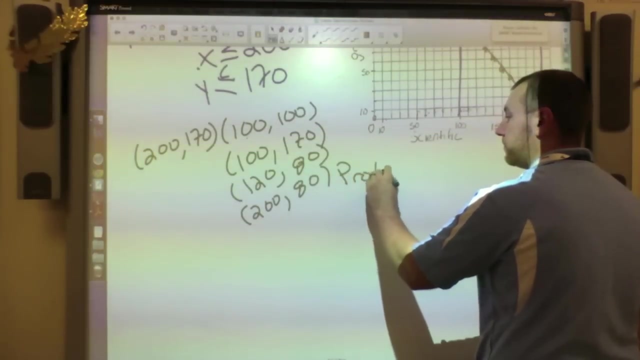 so I'm losing money. but graphic calculators produce a $5 profit. Okay. So if I'm losing money here, that $2 has got to be negative. If I'm gaining money here, that's got to be positive. So my maximizing equation, or my profit equation okay, of x and y: 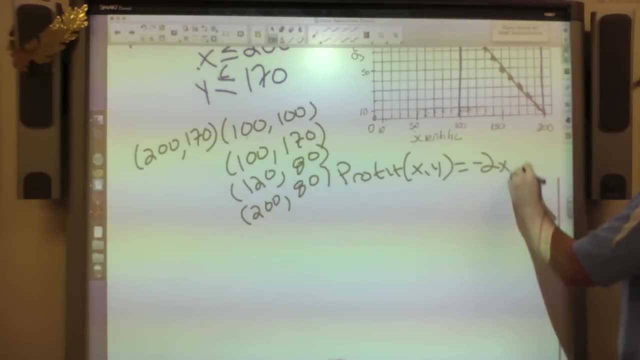 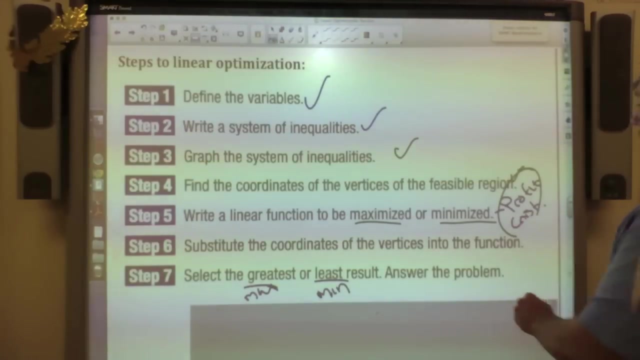 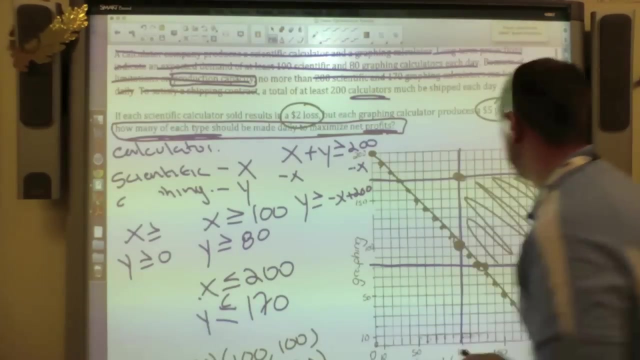 is going to be negative 2x plus 5y. I'm losing money for my scientific, but I'm gaining money for my graphic. All right, So that is a check. Now I'm going to substitute the coordinates of the vertices into the function, All right, So. 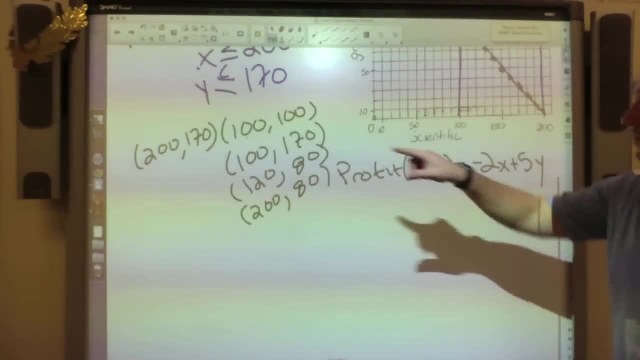 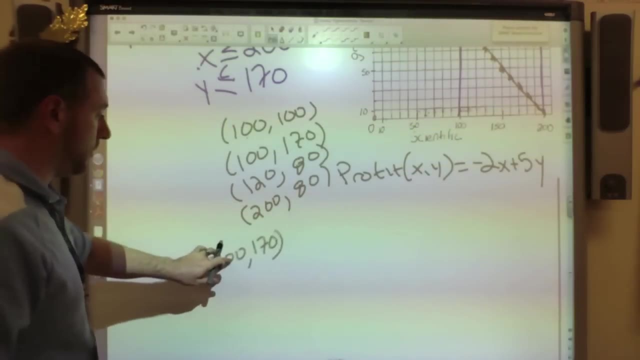 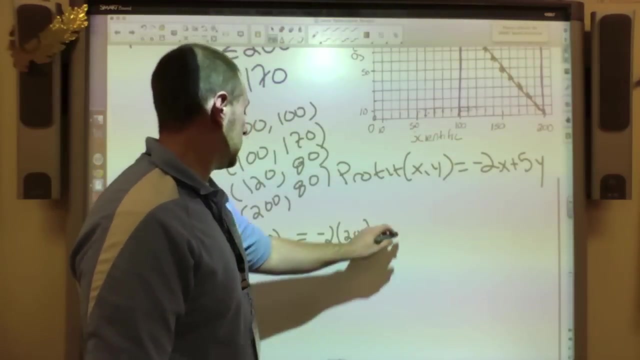 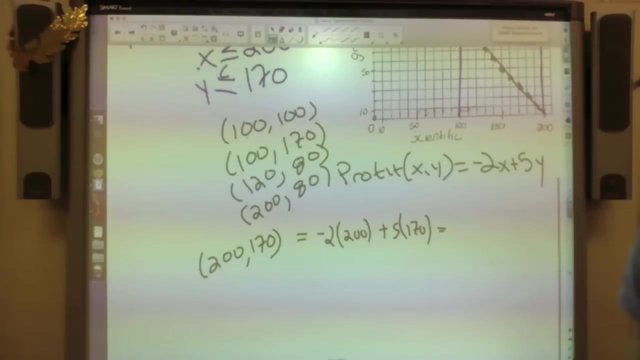 that just requires me to take all those points and plug them in. So, for 200- and I'll move this down. All right, That's going to become negative 2 times 200 plus 5 times 170.. All right, So that's going to result in. 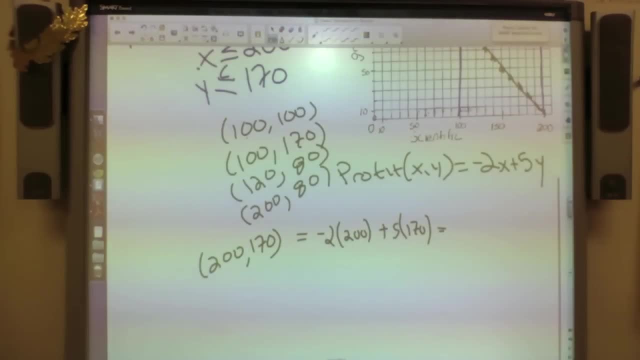 hit Uh, the drill room When By third. Good, I'll be done in a second, But if you need a room room I'll come and help. I'm just I've got to finish this up and then I'm good. 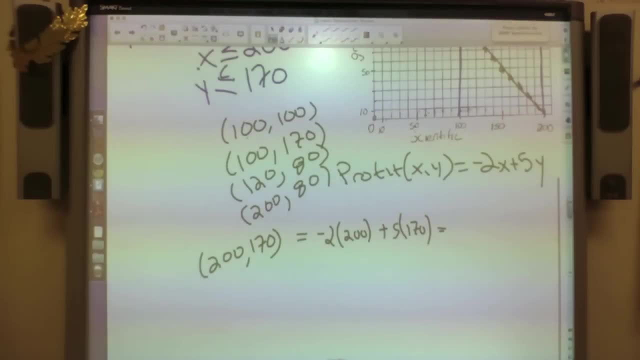 All right, This is going to be negative 400.. Okay, This is going to be 850.. So my total profit is going to be $400.. $450.. Okay For this one that doesn't want to come with me. 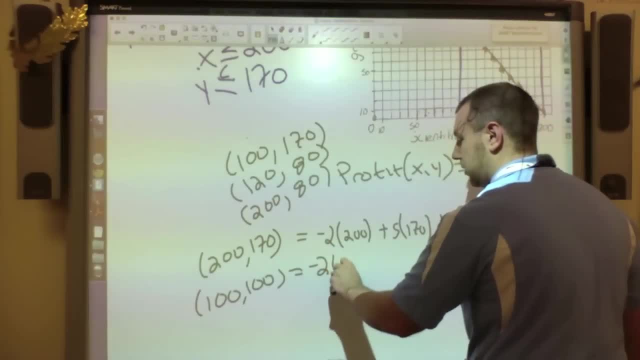 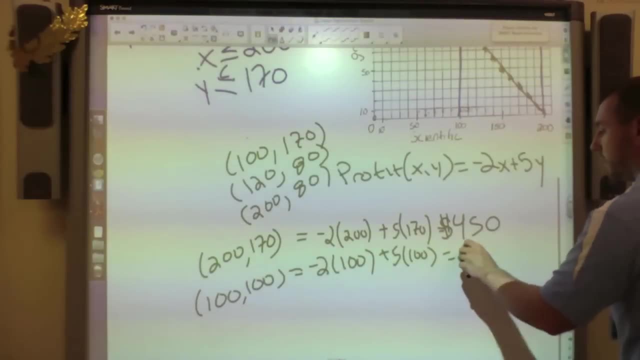 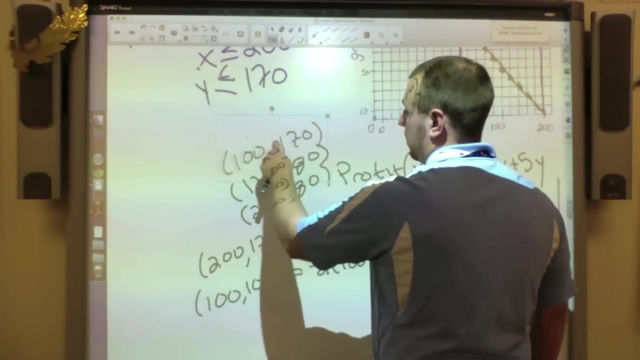 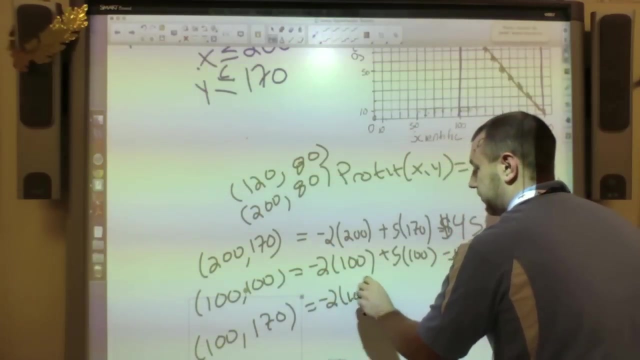 100, 100.. Again, negative 2 times 100 plus 5 times 100.. Okay, So that's going to end up being a 300 profit. All right, This, okay is going to result in negative 2 times 100 plus 5 times 170.. 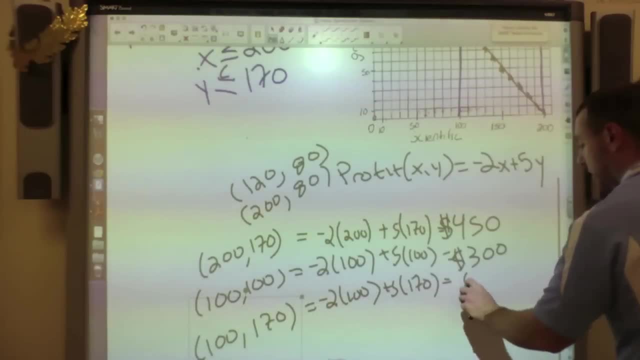 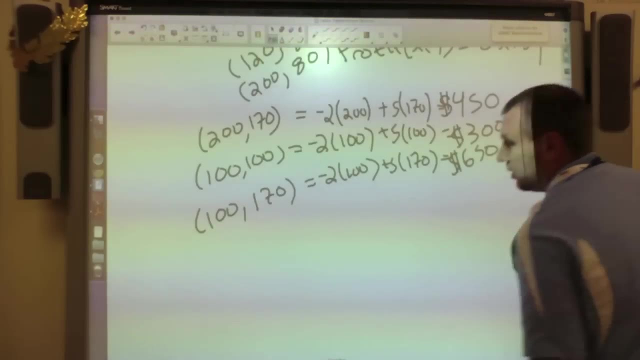 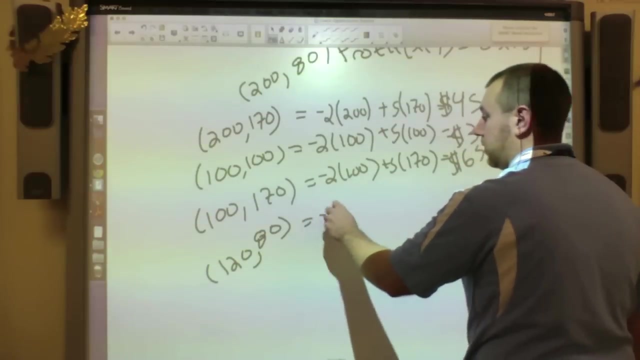 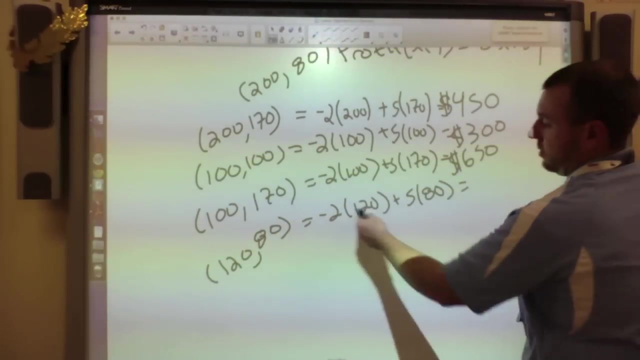 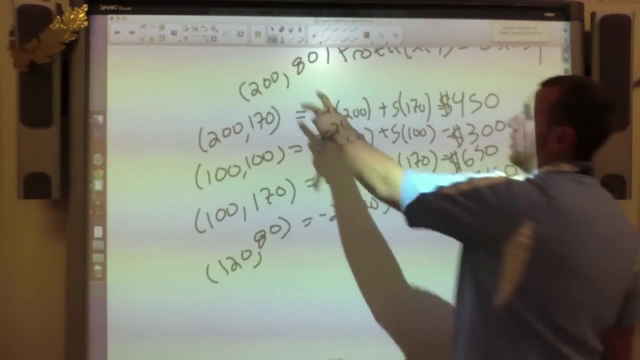 Okay, That's going to end up being a $650 profit. Okay, Negative 240, 400.. That's going to be a $160 profit. Okay, That's going to be end up being $650 profit Okay. 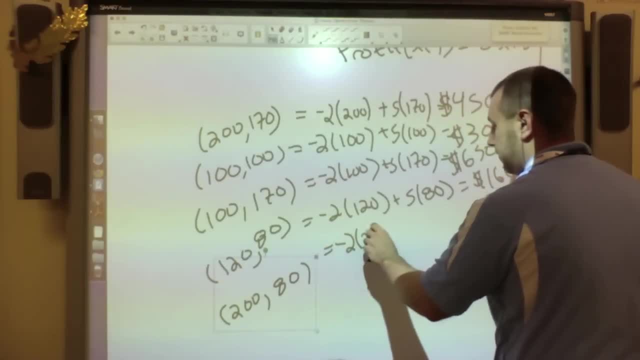 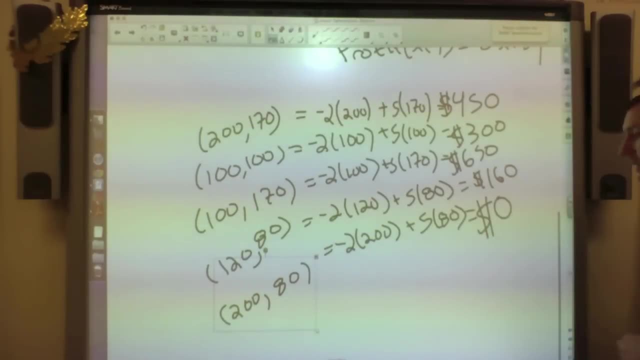 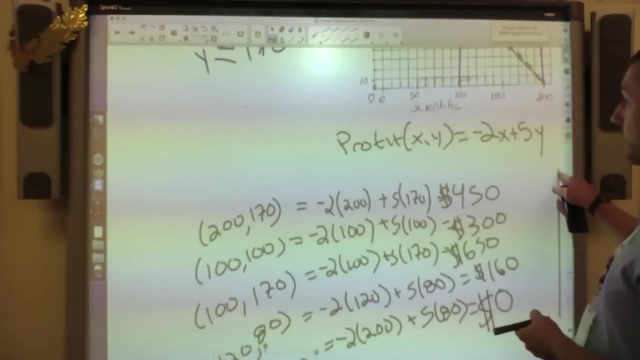 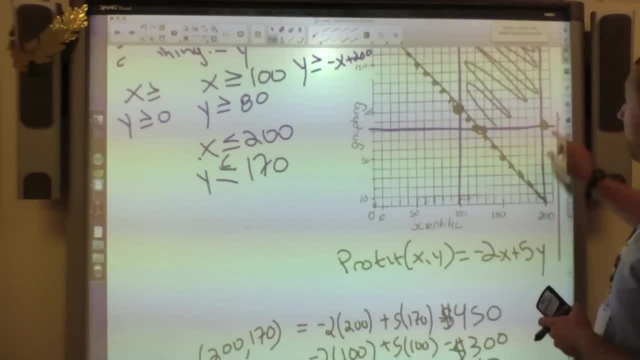 And this is all my profits, Right? So does the system make sense? All right. Well, if I'm losing something from my scientific, does it make sense to produce it more scientific or more of my graphic calculator? Well, if I'm making money on graphic calculators, 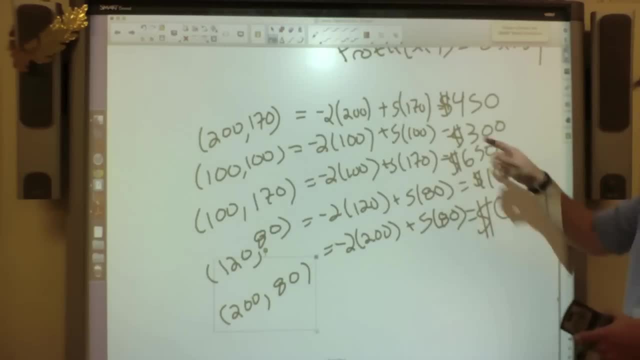 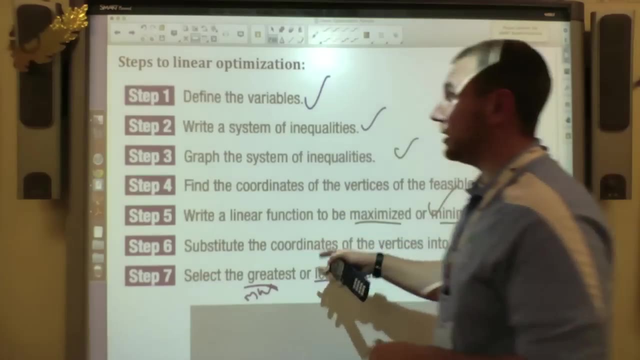 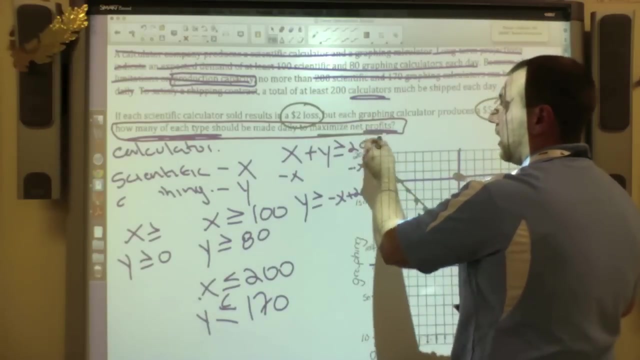 all right, so now all I have to do is go back and answer the problem. okay, it's like the greatest and least. well, what do I want to do? how many of each type should be made daily to maximize net profits? I want to maximize, so I want. 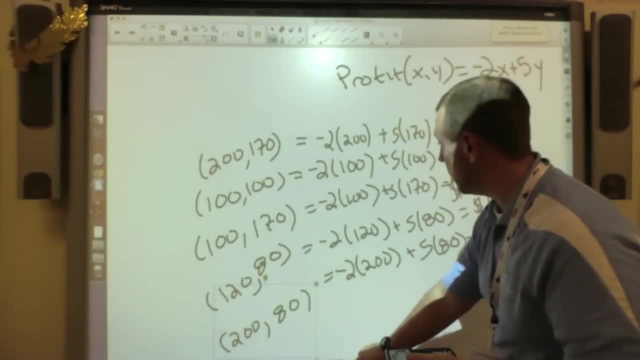 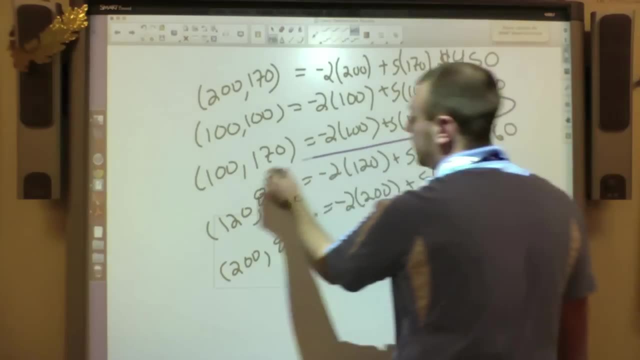 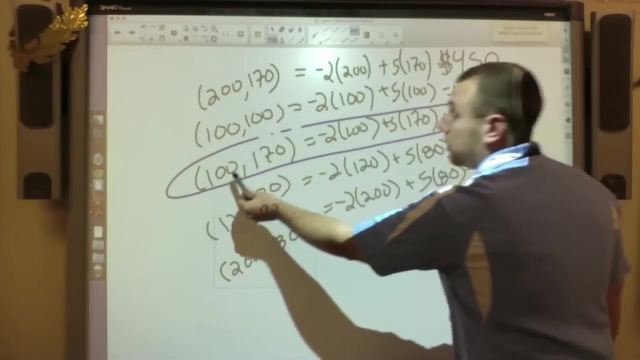 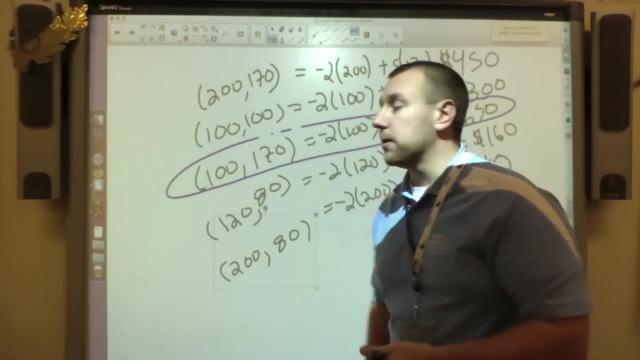 the total. okay, so I'm gonna continue going back here, okay. well, what's my maximum value here? oh, my maximum value is actually right here. okay, that's a six hundred and fifty dollars I make daily if I produce a hundred scientific and 170 graphic. it's not the point. now and again, word problems, it's never the.